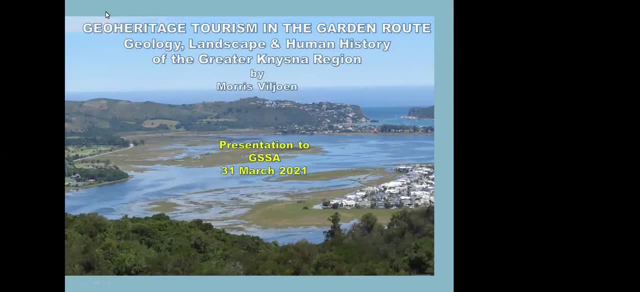 It's entitled Earth Link in the Kruger Park and that probably will be a topic for a future talk. But, Morris, with that you're going to talk today about the Knysna region in particular. Take it away, It's all over to you. 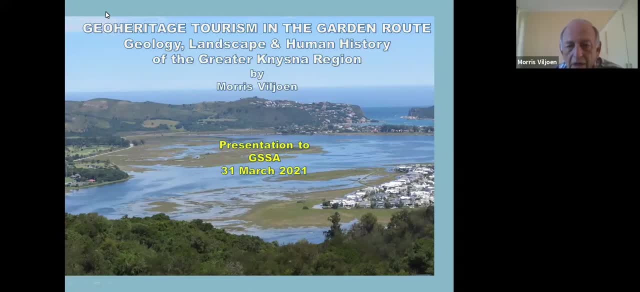 Thanks, Craig Noreen, for the introduction there. Craig, Yeah, Look, the Garden Roots is a well-known tourist region with a lot of attractions, Mainly the beaches. However, there's fantastic scenery there to be seen as well, like the lakes and the mountain areas and the valley and the gorges and whatever. 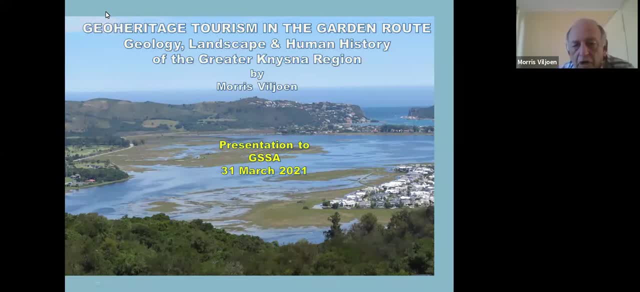 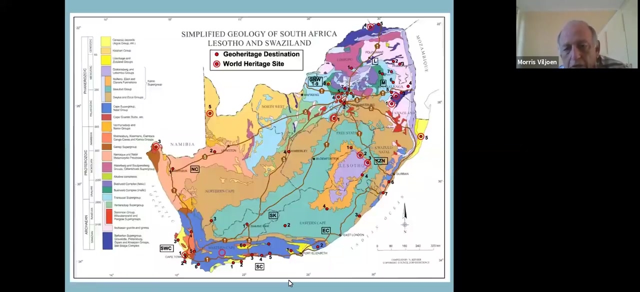 So this talk really concentrates on how the landscape was formed to give the scenic features that characterize the Garden Route today. I should just mention by way of introduction that it was even a project And to try And to try and develop geo heritage sites throughout South Africa. 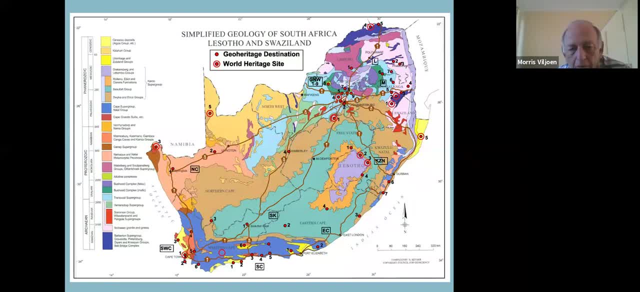 And we've come up with an initial listing of potential geo heritage tourist destinations throughout South Africa And they're shown on this map And you can see that 10 or 11 of them actually correspond to UNESCO World Heritage Sites And therefore those in any event should be the geo heritage sites should be developed. 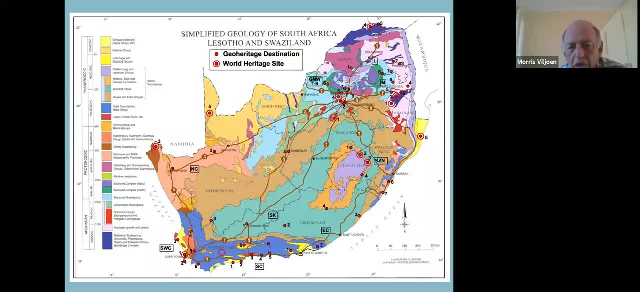 All of them have got some interesting geo heritage associated with them, those UNESCO sites. In any event, the site we're looking at today is essentially site number three there. Sorry, number four, But it includes a bit of three and five as well. 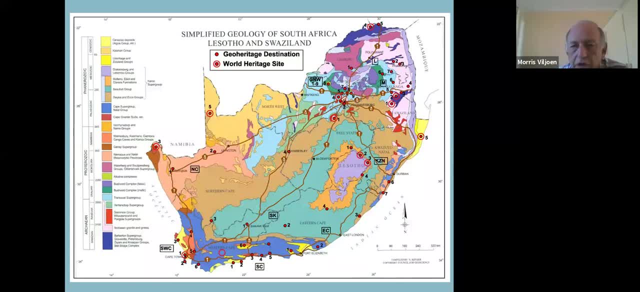 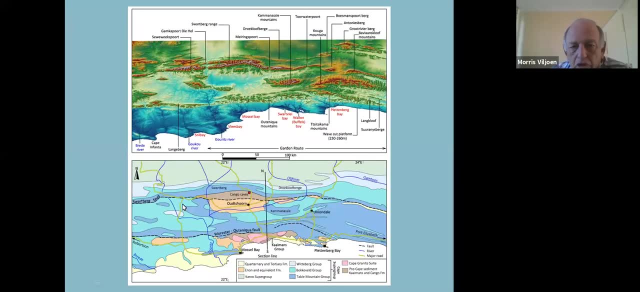 So it's essentially the heart of the Garden Route area. So, very briefly, digital terrain is always a useful thing to show What the area is about. We have the Cape Fold Mountains standing out pretty clearly to the north, And then we have the coastal plain, which is the light blue. 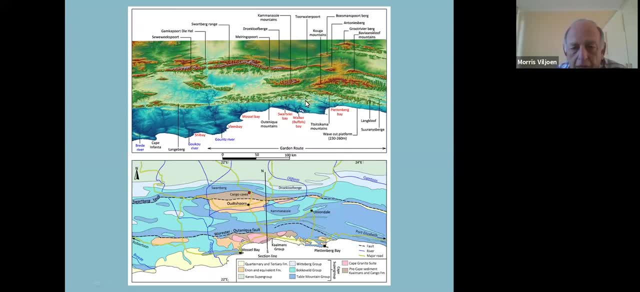 It's an old wave cut platform And that is incised by coastal rivers which drain off the Otunikwas here and off the Tsitsikamma here and the Langeberg over here. The only river that cuts through those mountain ranges is the Khoritz over here that cuts right through into the Otuswan Valley. 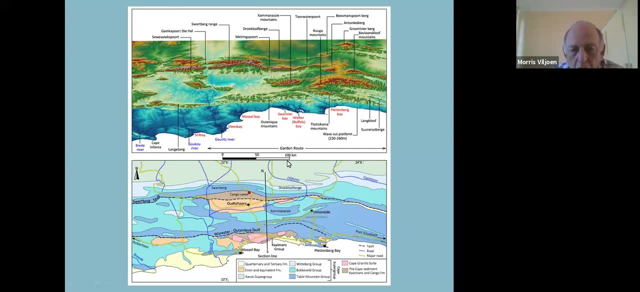 And then you can see the geology associated with that, Essentially the Cape Fold rocks, folded rocks. the Cape Fold belt is made of the Cape rocks with resistant courtsides forming the ridges. The coastal plain is mainly underlain by more ancient rocks of the Kaimans group, brown down here and then pink Cape graddits, very similar to what you see around Cape Town, underlying the Cape rocks there. 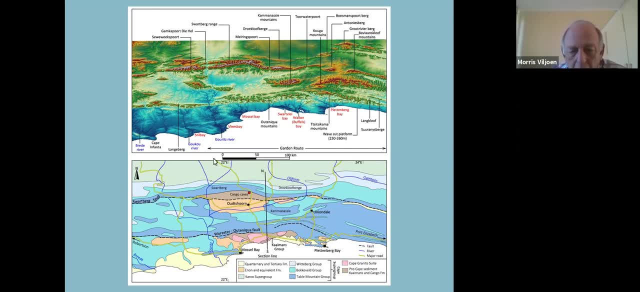 And then there are also some enon conglomerates which are Cretaceous age sedimentary basins, Mossel Bay area here, and also some Plettenberg Bay and a small area here around Knysna estuary. So we're going to really look at this region over here. 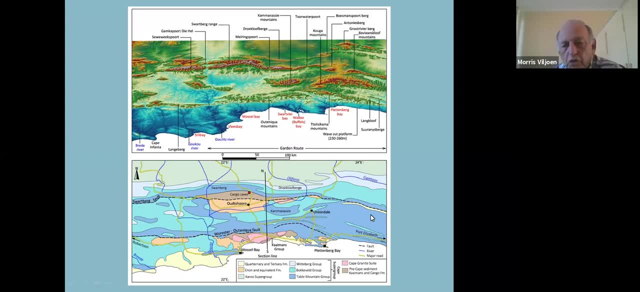 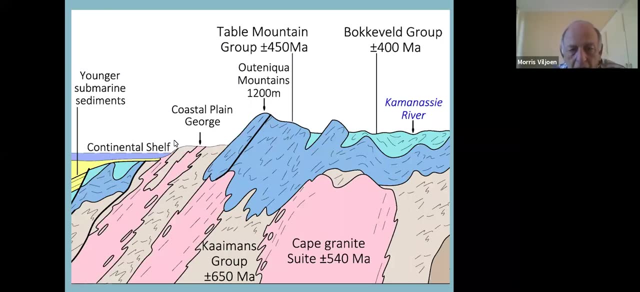 Cross-section is always useful as well to give some idea of how the whole topography works, And one here can very clearly see the coastal plain About 220 meters above sea level, And then of course the Fold Mountains, the Otunikwa Mountains, averaging about 1200 meters here. 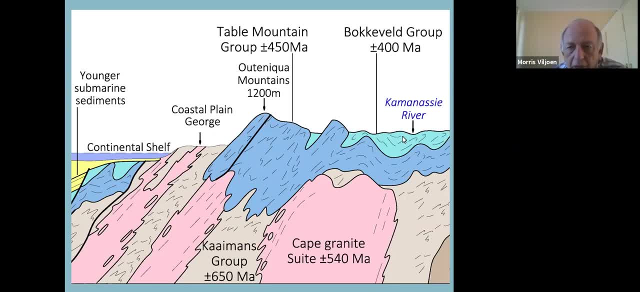 And then the Bokkerveld Shales in the Otunikwa Valley, in the Otuswan Valley. So we're really concerned with this region over here, the coastal interaction of these rocks and the coastal plain And the geomorphology of these areas. 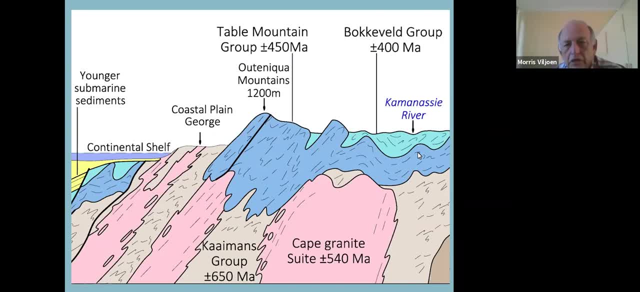 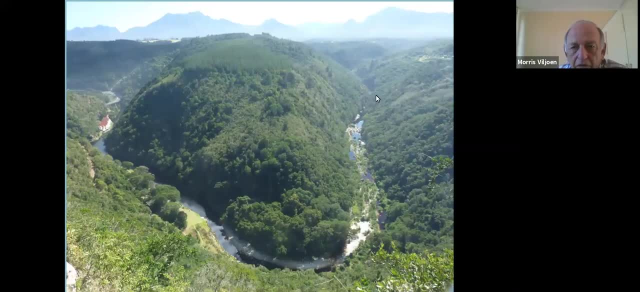 Okay, so here's the coastal plain being sized by the Kaimans River draining off the Otunikwa Mountains in the background, giving rise to a well-known tourist feature known as the map of Africa. And this is a view of the Kaimans sediments, well exposed. 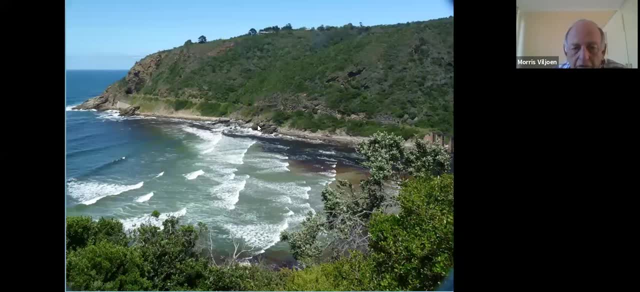 This is a typicality at the mouth of the Kaimans River And forming the coastline. here is a granite sheet, One of the Cape Granites, And this is exactly where the railway tunnel goes through. You can see the railway tunnel over there. 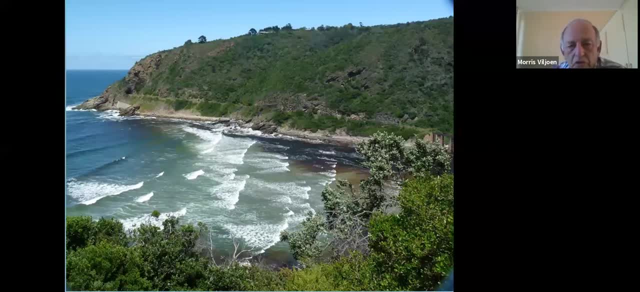 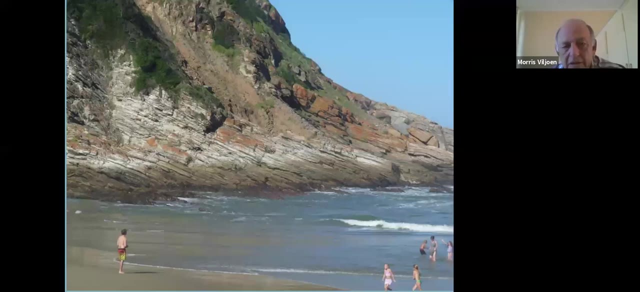 And they have the so-called Otunikwa Chuchu, a very popular tourist attraction in earlier days, But sadly that has fallen into disuse And here at Victoria Bay is a very good area where one can see these Kaimans sediments. 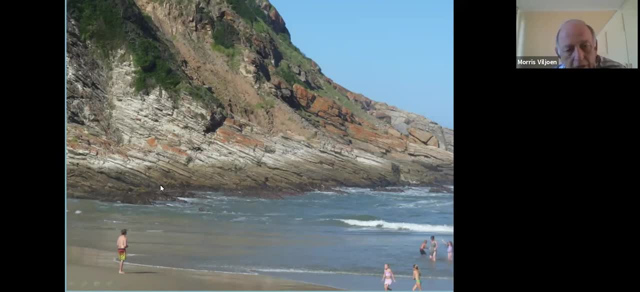 Essentially old sandstones with shalee, Shalee interlayers, now Sands and mudstones, now courtside and shale And overlaid by a resistant granite sheet over here. And then this has been breached by the sea and forming this nice sandy embayment of Victoria Bay. 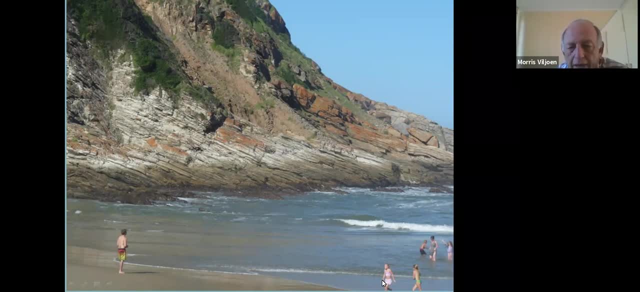 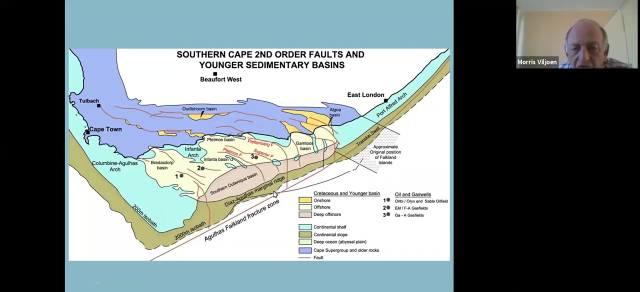 The only other embayment of that type along this rocky coastline is Harold's Bay, which is a very similar type of geological setting. And then, As far as the younger sedimentary basins goes, this shows the second order faults coming off the Gullis Falkland shear zone. 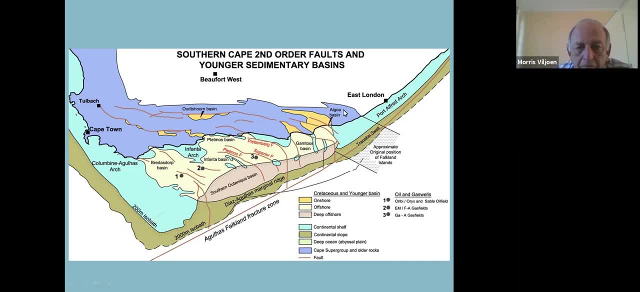 And trending parallel to the southern tip over here, And then erosion associated with this faulting resulted in these Cretaceous age sedimentary basins, such as the Otunikwa Basin and basin here at Plettenberg Bay and Mussel Bay. 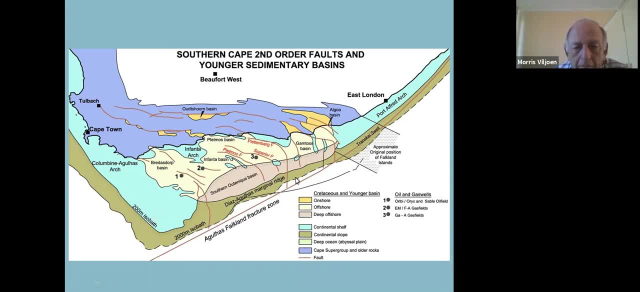 And, of course, the Algoa Basin over here, And at the same time, the coastal sediments formed, containing of course the oil deposits and some of the gas and oil fields of the southern continental shelf, And that's how those secondary basins formed. 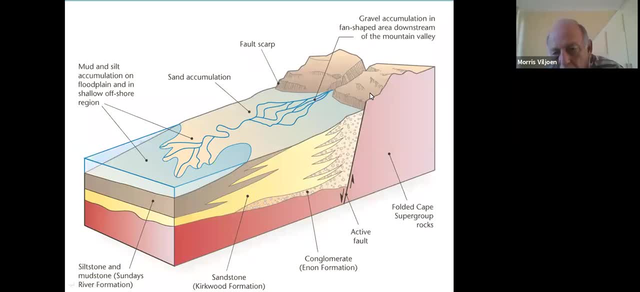 The enon conglomerates, of course, conglomerates joining those faults, turning into sandstone and then finally shale. This would be, for example, the Sundaes River and the Kirkwood Formation over here, And these would be the enon conglomerates. 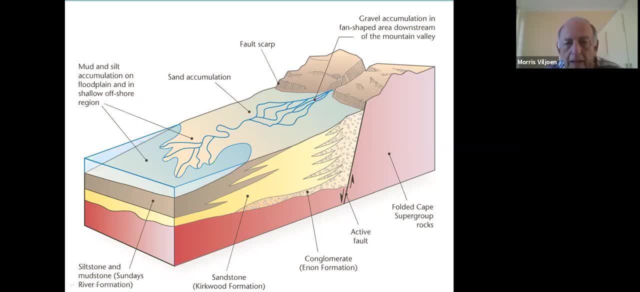 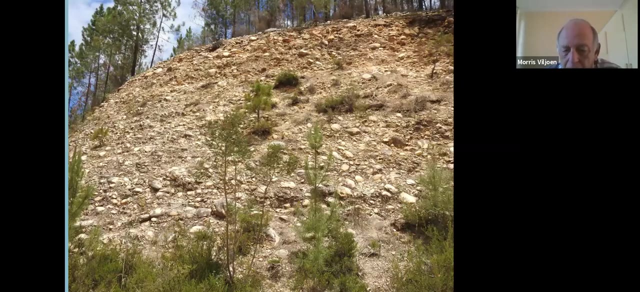 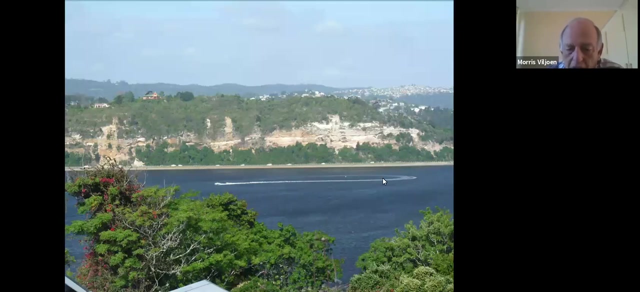 This is how they formed. Another example on the Phantom Pass around near the Knysna estuary: Very coarse conglomerates just shed directly off the upfaulted side of the fault here And then also very well exposed enon conglomerates On the north flank of the Knysna estuary, well seen over here. 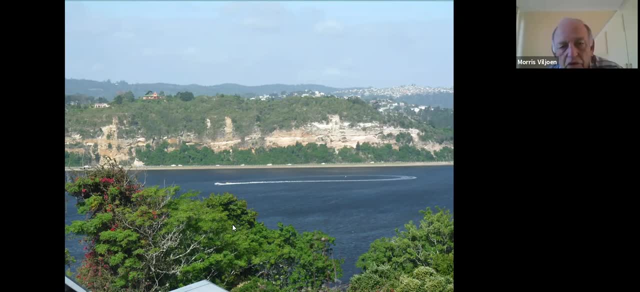 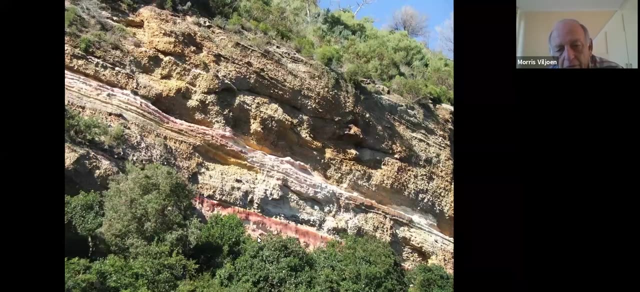 And this gives a good idea of what you see. these conglomerates And interlayered sandstones often pretty colorful, as you can see here: Reddish and yellowish and white sandstones with interlayered conglomerates. This is really close to the proximal area of the enon. 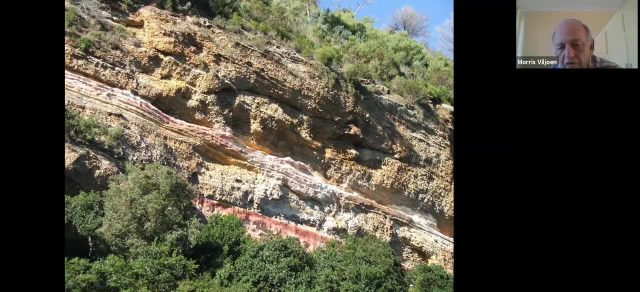 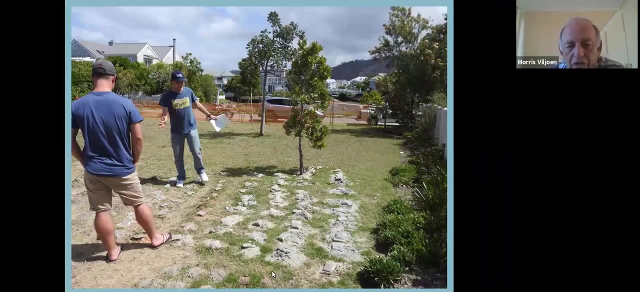 But as we get into the Knysna estuary itself, And of course Not exposed, because they're less resistant, rocks Are in fact more shale-type rocks and fine silts and shales. So Willow Steer did this, drilling over here. 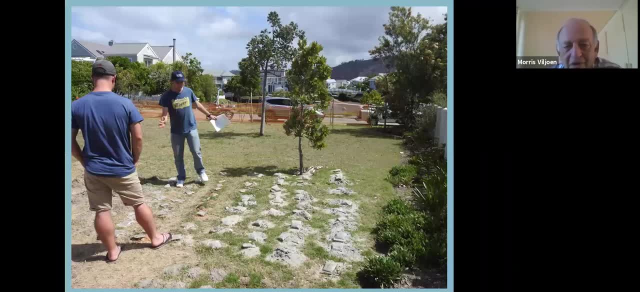 They're looking for water in what they hope to be Peninsula Formation Quartzite But turned out to be a proximal area of enon conglomerates. Softer cinnamon shale-type things with no water in them, And then an important feature is the so-called wilderness embayment. 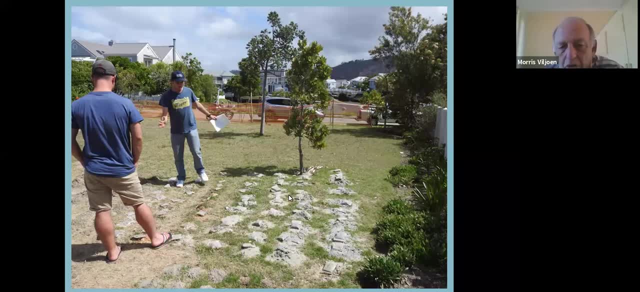 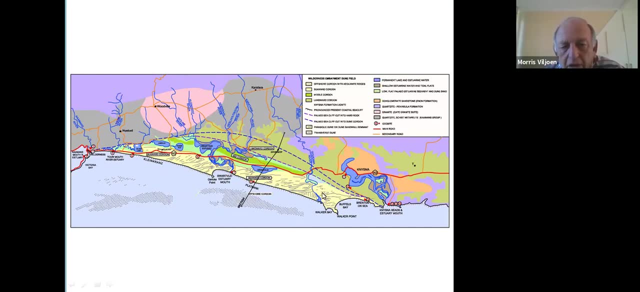 Of which there are four main sand cordons or belts. There is an offshore cordon over here, Not far below sea level in places. Then you have what is called a landward cordon, A middle cordon, mid cordon, the green- 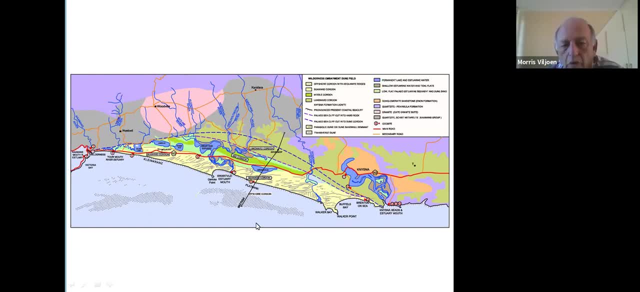 And then the khaki color is the landward cordon. This mapping was done by Illingberger And it's taken from his map Sort of of the area. The other thing to notice is that in between the cordons You get these shallow areas of sort of estuary and other. 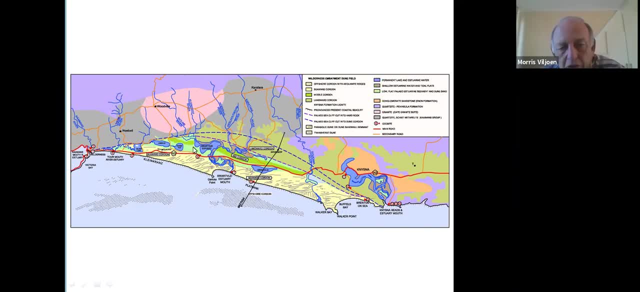 The Custrine deposits Where the lakes, the famous lakes of the area, occur: From Island Lake over here To Long Flay, Rona Flay, Swat Flay And then Kryn Flay over here And Rake to Flay in this valley over here. 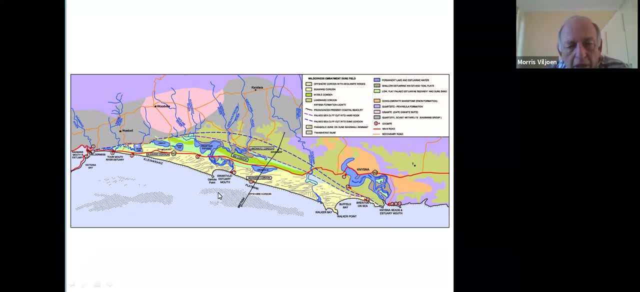 So that is quite a feature of the area. The cordon has been breached here by Swat Flay, the mid cordon, So that occupies the area where the mid cordon could have been. A remnant of the coastal cordon is preserved in a place called Island Lake. 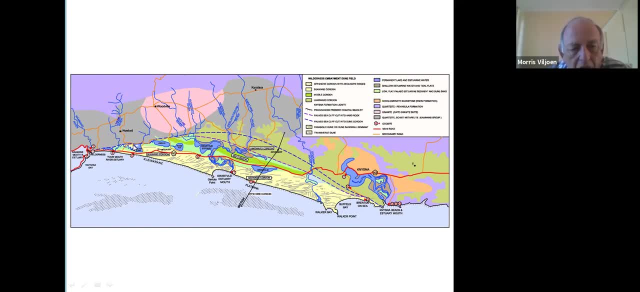 This is the island And the meandering river. In the flat area it joins the Toe River. That's the river that exits Wilderness Is called the Serpentine for obvious reasons, And these, incidentally in red, are the stops on the excursion that. 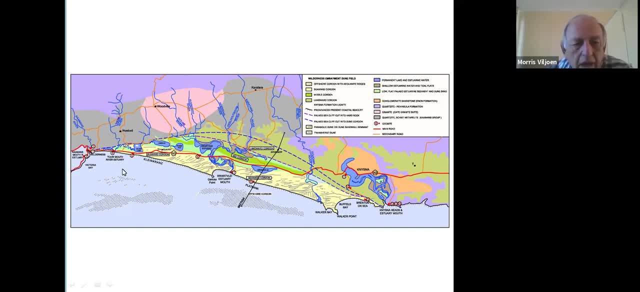 On a several occasions now, The about 14 stops All along the coast which highlight All the features I've been talking about. And the other feature of note Are these embayments, Buffalo's Bay over here, And the embayments all. 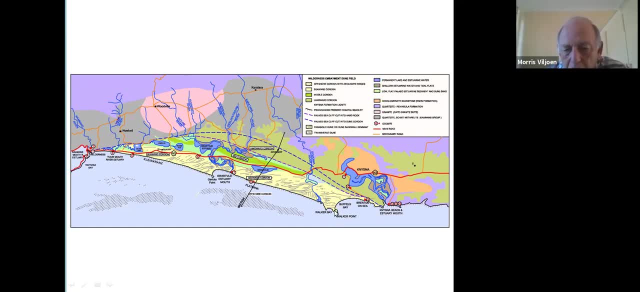 Occur behind resistant Ridges or points Such as Walker point here, which is actually a piece of A table of TMS, a peninsula court site, Walker Bay, Also a little peninsula of court site here. And then there's 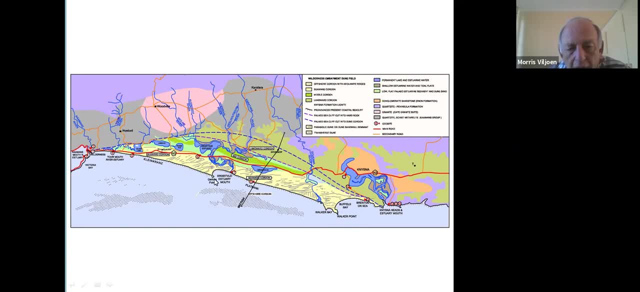 Another one here called Swat Flay Estuary And that that little Promontory. there is actually a very Resistant piece of calcified dune rock And then Yeah, So those those are some of the main features. 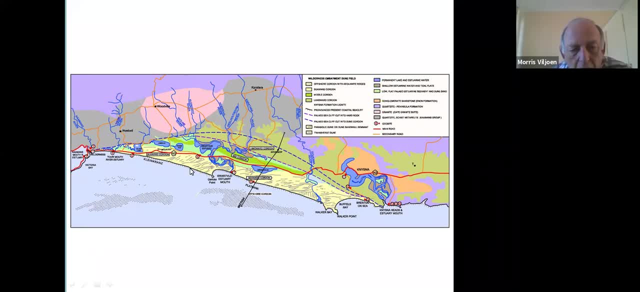 These Embayments and then in between, These are coastal cliffs, but all made of calcified Land, Sorry. And At the place to see the, Or the older rock formations is here, Victory Bay. I mentioned that over here. 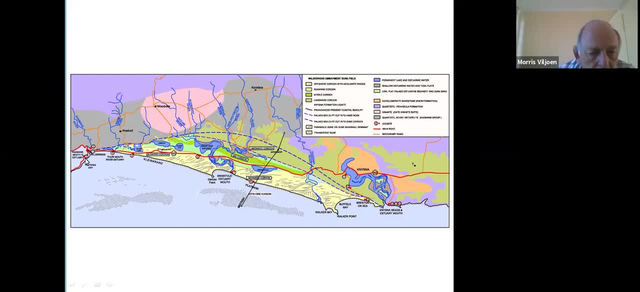 And, yeah, Victory Bay. Yeah, Over here, Victoria Bay. Okay, So then the next one is a cross section through there which gives Also a bit of idea of What these corns like. So there's this Seaward cordon. 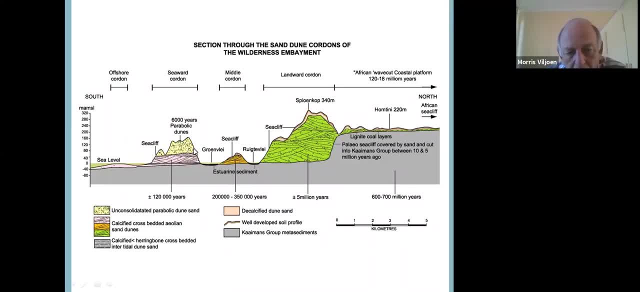 Calcified tips that I mentioned, But then overlaying by much younger Parabolic sand dunes. They only a few thousand years, These things. And then, And then The calcified dunes here: 120,000.. In between this, 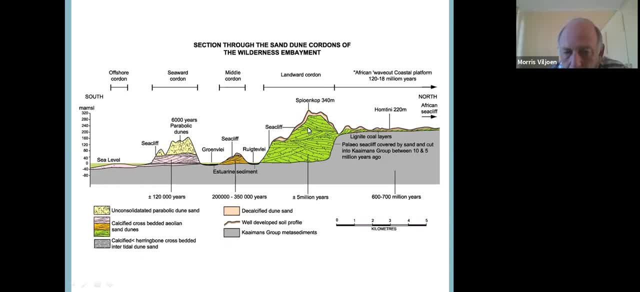 And the mid June cordon And then the land of June cordon, Quite a significant accumulation of Of June sand, With a really high point here Being a notable feature, And that is well above the actual coastal plane. It does overlap onto the coastal plane. 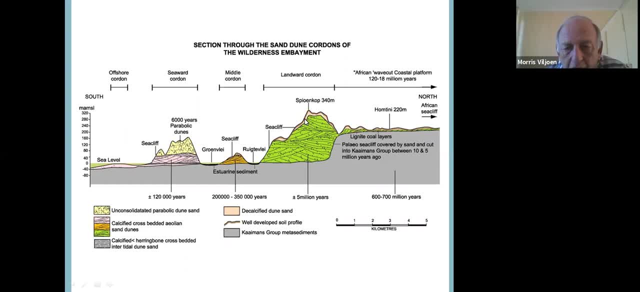 And significantly it's got quite a good, Well-developed soil profile on the top, And so has the middle June. But these younger parent Bollock dunes have got no real soil Profile, is still essentially June sand, So the vegetation on these is really sparse and scrubby. 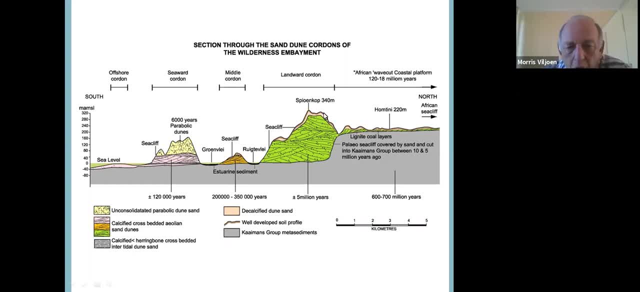 And not just shallow rooted, Whereas here Plants grow very well, forests, And of course There's quite extensive forest station. It's taken place On the land With June, as well as on the mid June as well, Right. So here we see some of the land with June. 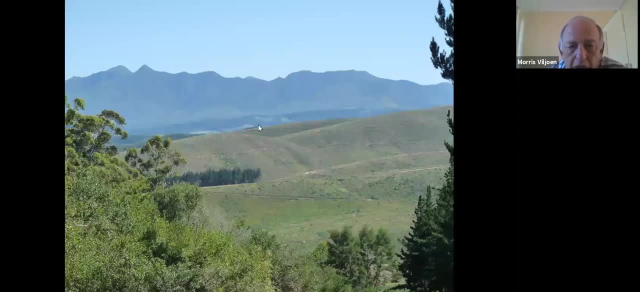 Overlapping onto the coastal plane in the background with It was in the background. And here is another view Of the land, with June And here it's overlying in on conglomerates. This is on the south flank of the Nice in the history. 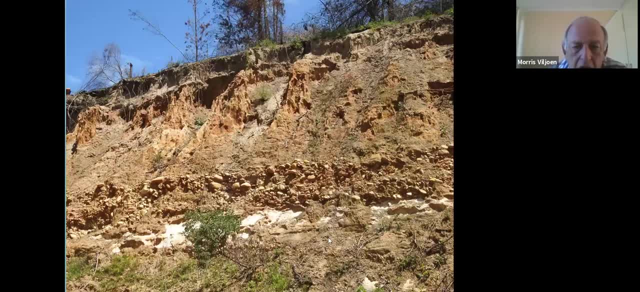 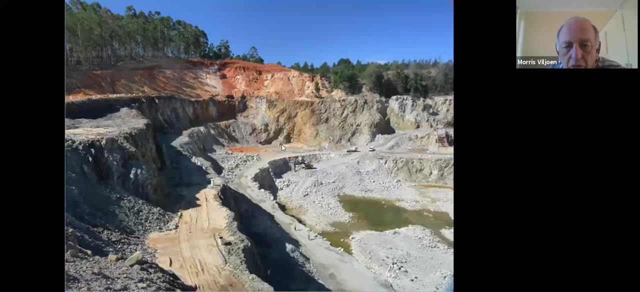 Overlying in on Conglomerate and sandstone And you can see it nicely developed soil profile on the top of the land with June, Yeah, And you see the same thing here in a quarry And this could be in Ron quarry of the folded. 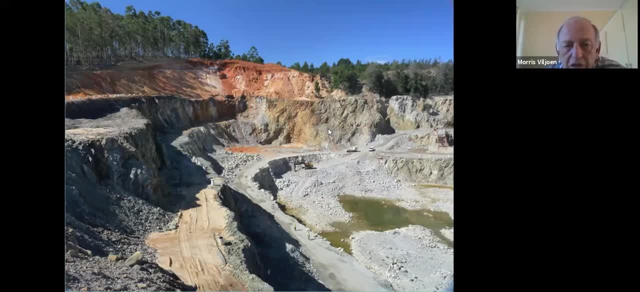 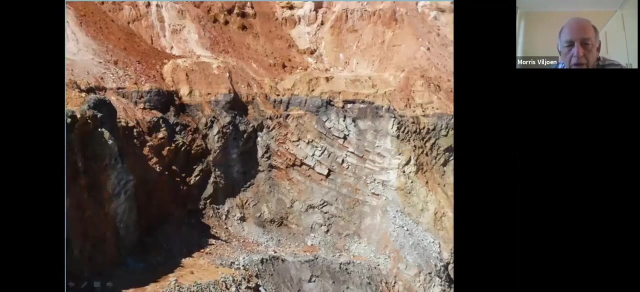 Table mountains, sandstones, But there you can see the overlying June Well-developed soil profile and forest growth. And there is that contact interesting on on that basis. Contact Is a is a seam of lignite or brown coal. 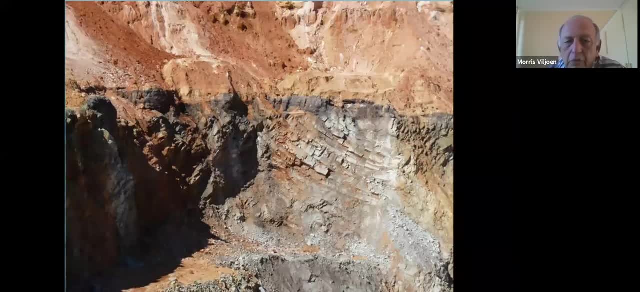 And And that formed when you must be in sort of a marshy condition on the old high standing coastal plane, possibly a remnant of When the the sea retreated, Marshy conditions and lignite Cold formed, And that was then overlaid by the sand June. 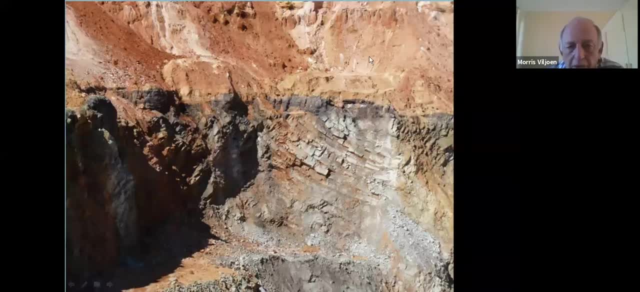 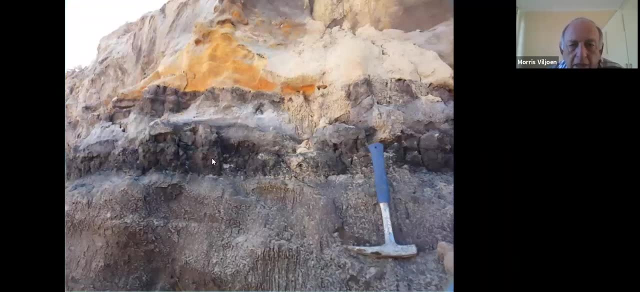 which is dated at 750,000 years, The land would send you. And then This is multiple Lignite Seams at this locality, in that That's exposed in the quarry there, And this is typical of those dunes rounded. 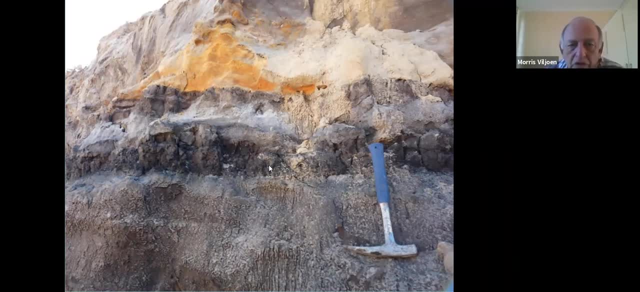 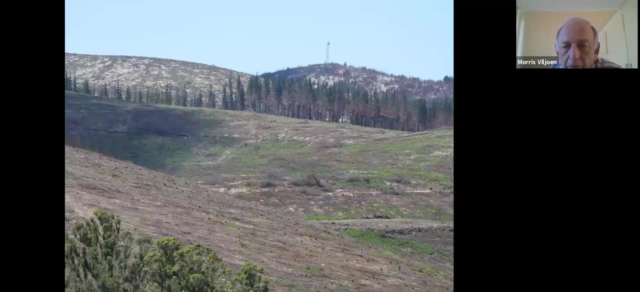 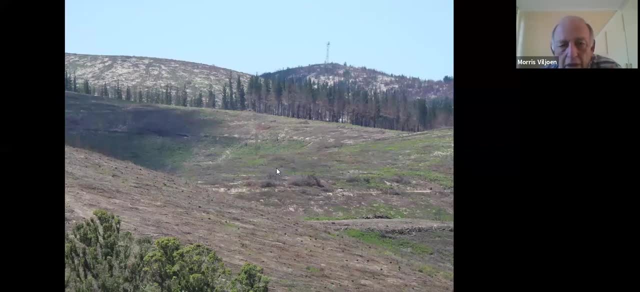 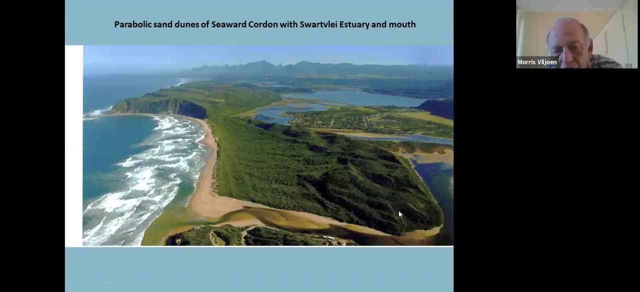 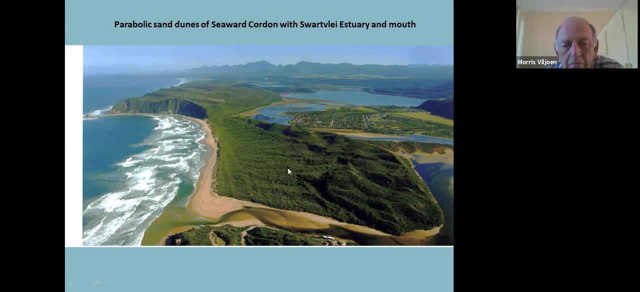 This is a parabolic divisions here. This is actually Transverse dunes coming at that direction. I bet it's maintaining parabolic dunes that you see, well developed in this region, Overlying The older calcified dunes which are well-exposed. 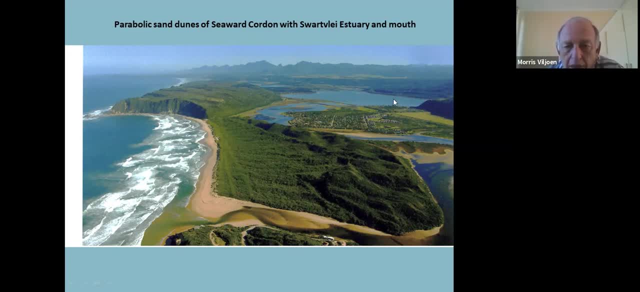 Yeah, These carrying a point which I mentioned earlier, So getting a classical little abatement here. This is one of the extremes: flowing around what is called the island here and then meandering through here and finally cutting through the land and see what dune field here. and this is the swat ray history mouth. 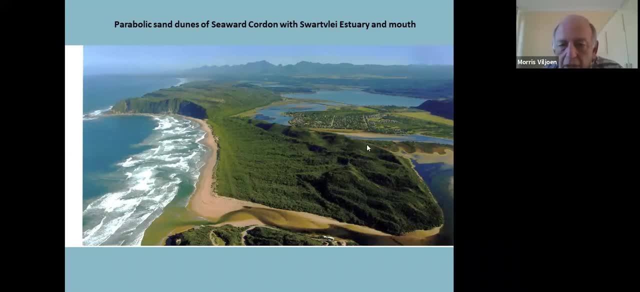 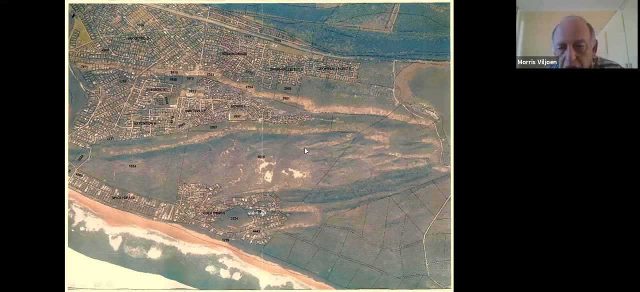 there are the parabolic dunes, which you can see quite nicely on the google image here, where he's clearly deposited, with wind from the south, uh, west, southwest. and these are these parabolic, uh closures of the of the parabolic dunes, with the, um really, or the threadbare vegetation on. 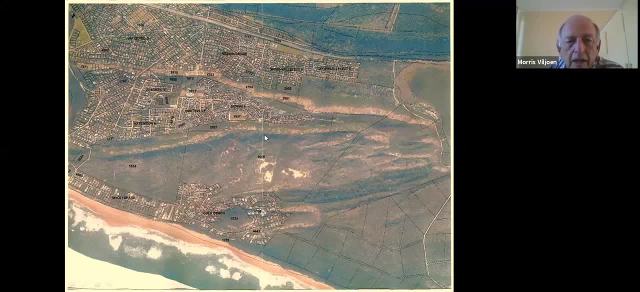 the dune faces like this face over here and this one here. so this is the northern flank of the seaward, younger seaward dune field and this is the interdune valley and mid dune here with covered by good forest vegetation. so there is again the scarica point in the 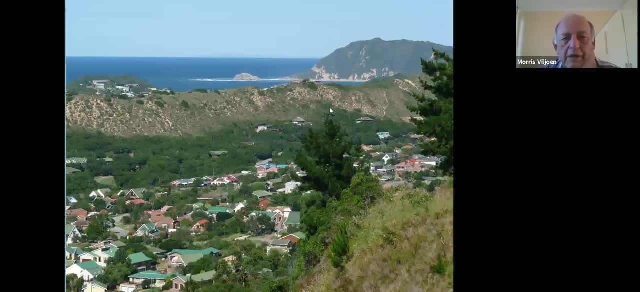 background with calcified dune rock and then overlying younger parabolic dune field. it has the northern flank of a parabolic dune really threadbare, and however, at the base of those dunes you get some very nice development of milkwood forest due to, i suppose, nutrient. 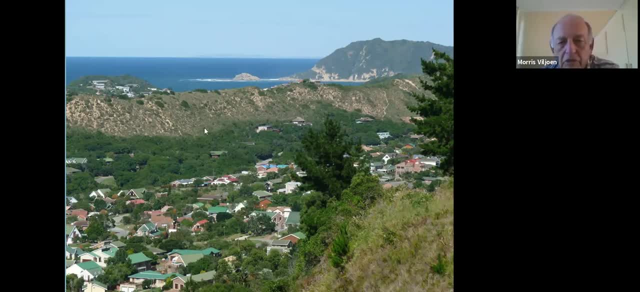 and finer grain stuff that's accumulated at the base of the dune. here and this is the interdune valley between the the coastal and the mid dune. the photo taken from the mid dune field just above, overlooking some of crune play at search field. 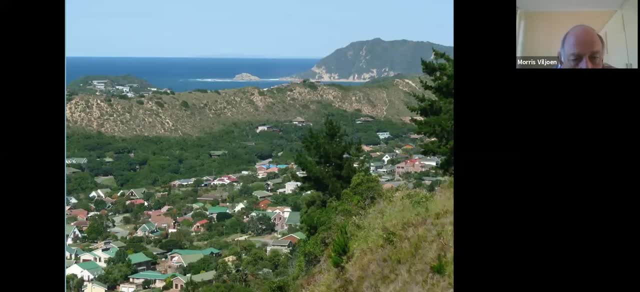 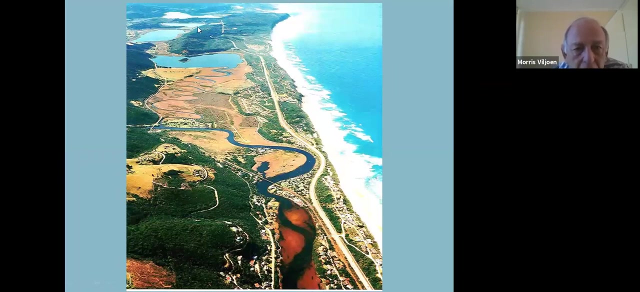 in fact i'm sitting right at the moment there. i'm right, right there looking out of that window. so this in fact shows i mentioned the island lake and you can see the resistant dune here. it was a little remnant forming the island and then you can see. 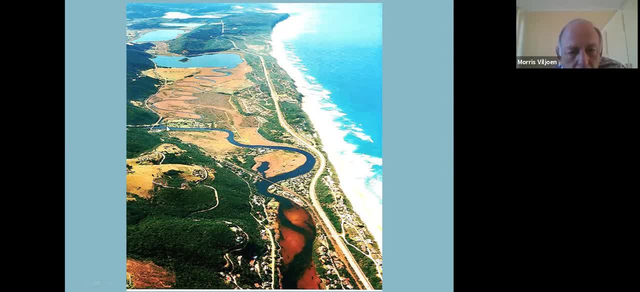 serpentine river winding its way through, joining the toe river, which is the river that runs through wilderness and exits over here. look at the mini estuary and um yeah, so that's good. and near the other lakes in the background it's a long flay, ronald flay, swat flay. 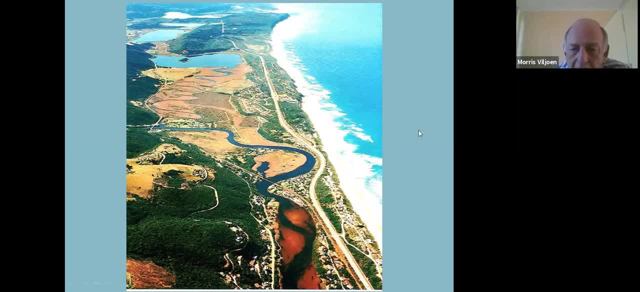 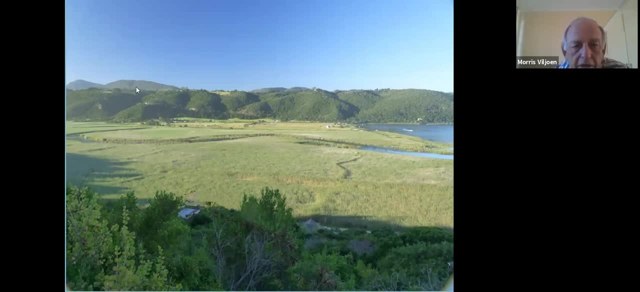 so this is the point where the serpentine exits island lake and you can see it winding around through here. the background: this is an old sea cliff and that is the um, the old coastal plain up here. so here the the rocks here are essentially alkaimon's group and granite material, quite resistant but definitely an old sea cliff. 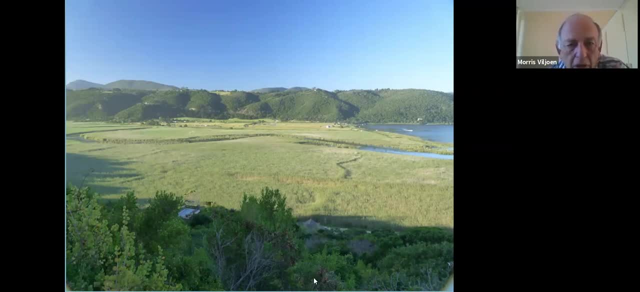 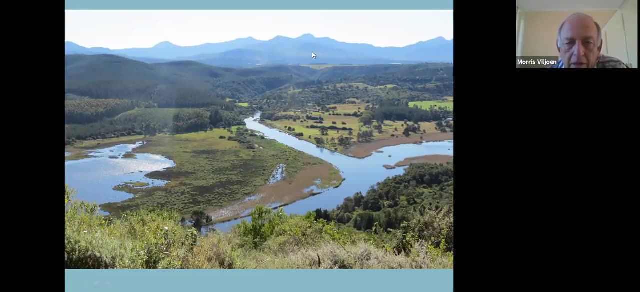 and another example of uh we're taking: from the mid dune looking towards the land, with dune cordon, the coastal plain and the otanique was in the background, you can see this karatari river has cut a gorge, mini gorge, through the edge of the. 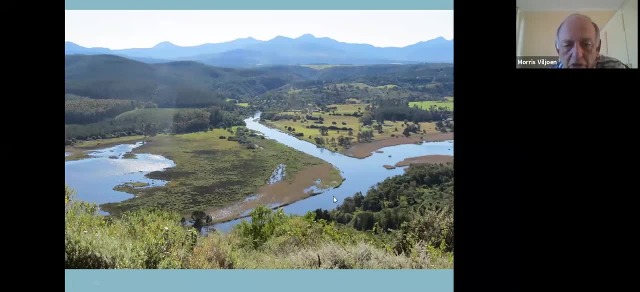 old cliff face and exits here at a place called rector flay, which is between the mid and the landward dune cordon. it's a part of rake to flame in the karatari river and notice the forest growth over here. um, okay, um, and these are typical calcified sea cliffs. 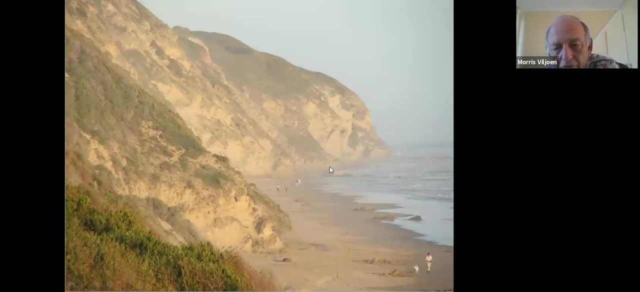 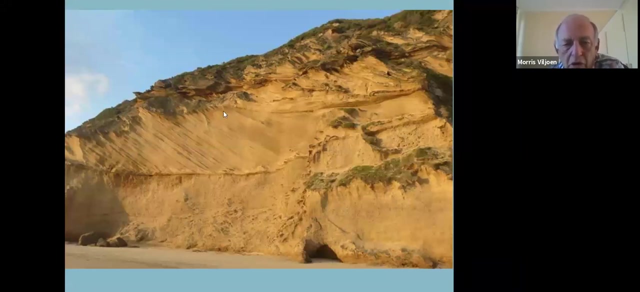 near a place called prutt bunk. there is often a bit of a sandy beach, but sometimes the cliffs are pretty resistant and there's not much to beach and uh. classic examples of these calcified aeolian dunes: large aeolian dune form. various types screamed forma calcium continuous. 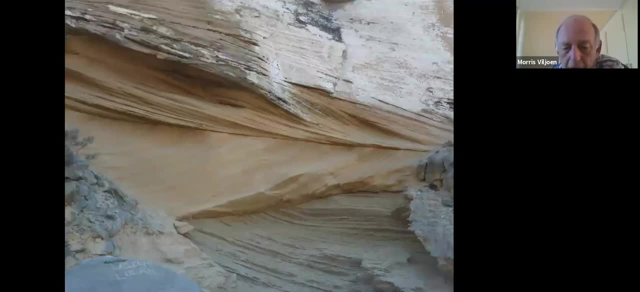 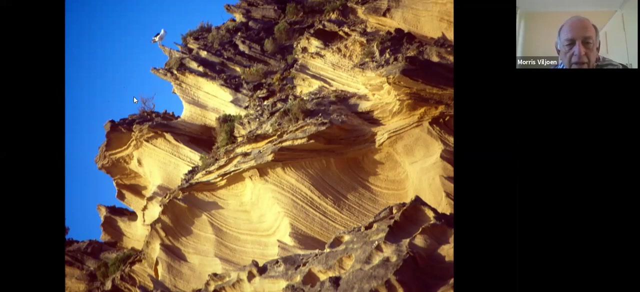 some more examples. these are from brenton- okay, an absolute textbook: typeuna sea cliff, aeolian dune, sand, but calcified. Some more examples. and of course, birds breed in these areas and a whole range of very interesting seabirds occur: seagulls and 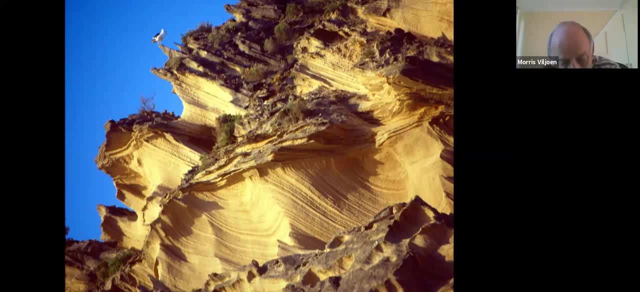 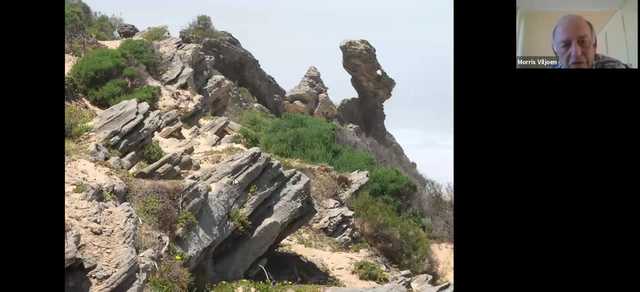 I forget the name, but anyway- and some interesting sculptures occur here. these are calcified cross beds, dune cross beds, and he has the head of an Egyptian mummy, or Egyptian pharaoh, I suppose you could say, at sea level and below the aeolian dunes, aeolian dunes- here you get the. 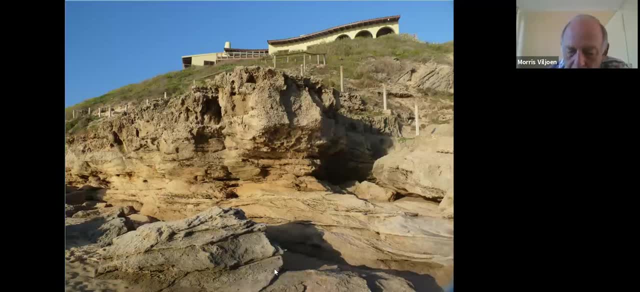 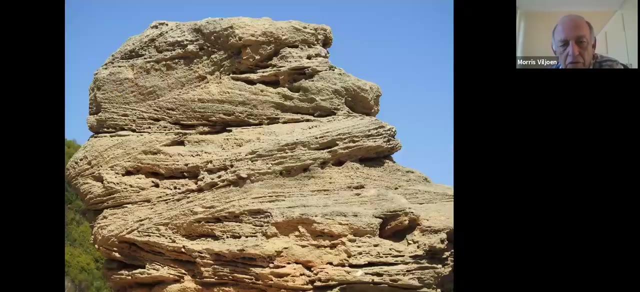 these herringbone type cross bedding, which is planar beds, but then with herringbone type in between, as you see here, and this herringbone dune material is typically developed where you have tidal forces of incoming and outgoing tide. so these are now tidalites or calcified paleo tidal sediments at the base of the aeolian. 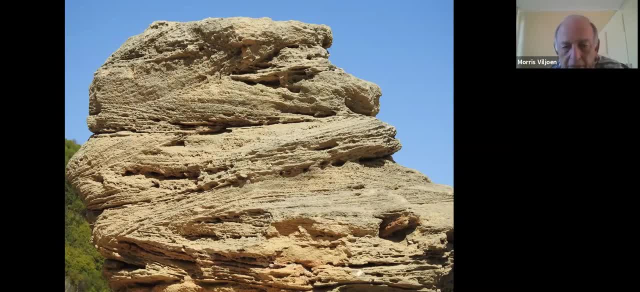 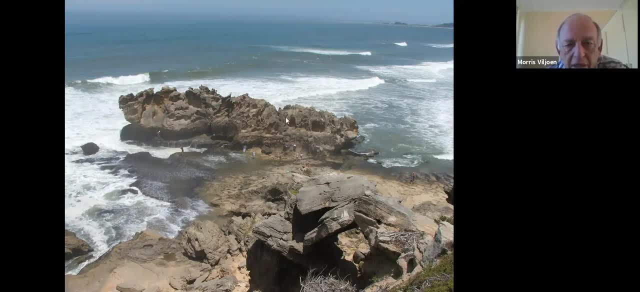 calcified cliffs and that is this castle rock. I think I mentioned well this castle rock. I think I mentioned well castle rock at Brenton, very resistant, but you can see how it's being eroded here, here, and these are all tidalites at sea level and some of these also old tidal, calcified tidal. 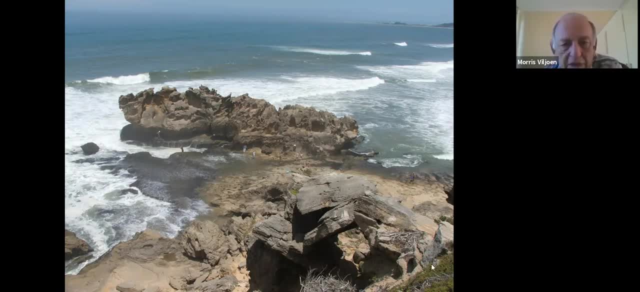 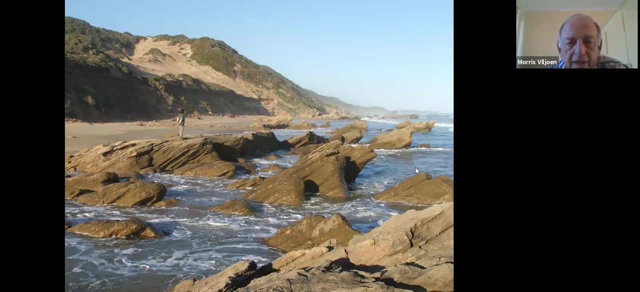 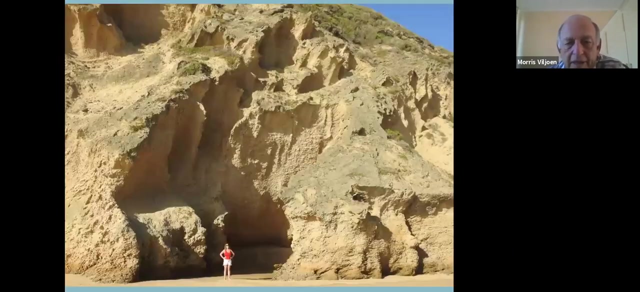 deposits here as well, these forming a wave cut platform, but very resistant cross beds, in this case preserved on the coast. here, however, in many areas the calcification is very terrible and you're getting areas of lower calcification which have been subjected to preferential erosion. as you can see here, some fairly spectacular cavities have formed. 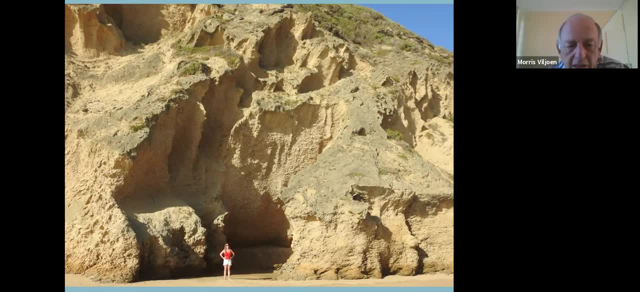 in these sea cliffs where the calcification hasn't been as intense. the calcification, incidentally, coming from dissolved lime, from sea shells in the overlying sediments, a dune material in the overlying sediments, a dune material- has been deepening the calcification institution. 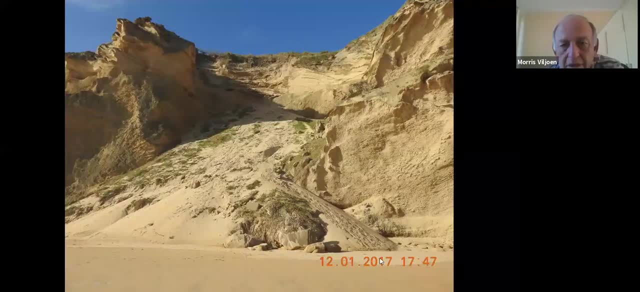 there are some small little vicious cogs here, but I'll just do a quick look at this. that's one of the ones that we have still in existing pieces in the area of the calcification system. this is one of the first or very recent land slides. that we probably took place in about- well, the date of this photo is 2017.. about 2060- yeah, end of 2016- and I had a look at these a little while ago. there's some definite footprints or foot imprints. some definite footprints or foot imprints. I think they were made here here at the San Francisco. 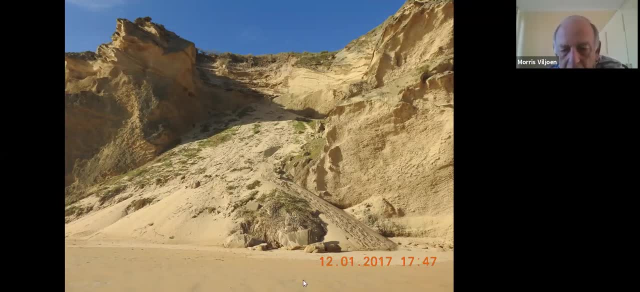 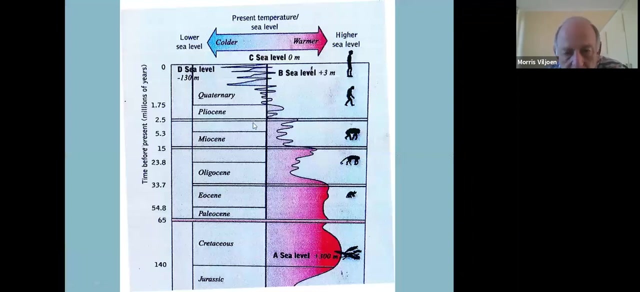 prints of animals and other imprints of early humans who were in the area also been found and this actually shows the different sea levels due at and different temperatures. over time you can see there have been dramatic changes of sea level and temperature and sea level um going back to cretaceous times and eocene prep and the paleocene in the oligocene, when 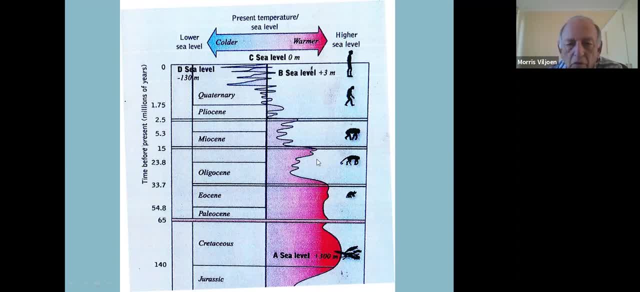 you had some pretty high temperatures and then it's fallen off to modern times, but with minor fluctuations throughout here, and each of the dune corns i showed you was at the base of one of these sea level changes. okay, the face of the dune cordon formed the the coastal cliff of one of those. 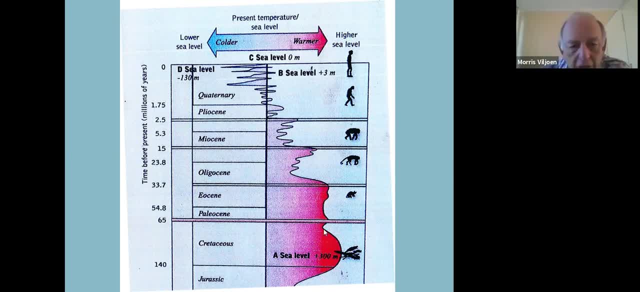 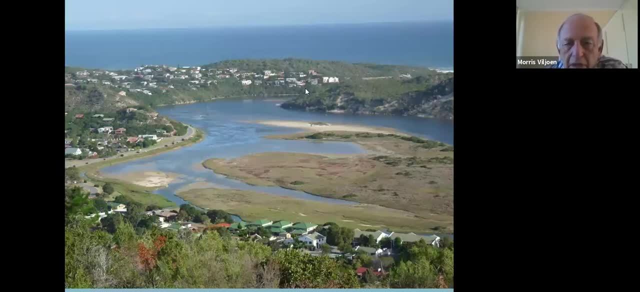 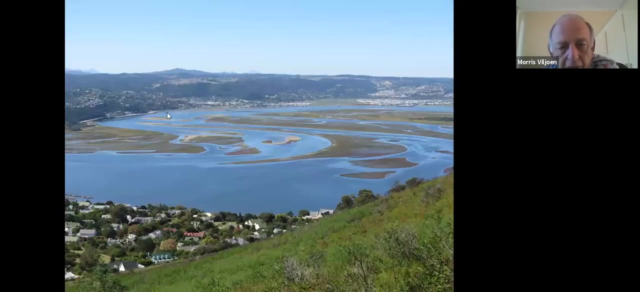 sea level changes. there's another estuary, um, the, the swat flay estuary um, which exits here through cuts through the, the land, the, the seaward dune cordon and exit at swat frame mouth. and then another estuary, well known, of course, is the neisner estuary, with some classical meanders. 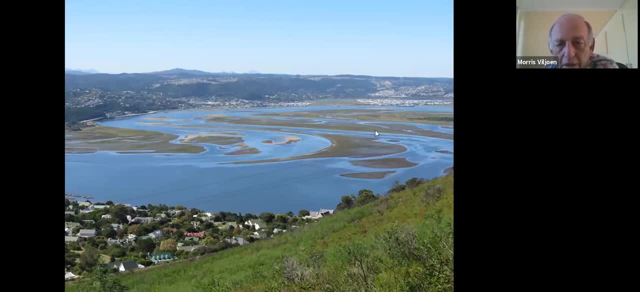 underlain by um, as i mentioned- and that's a very interesting thing to have in the past- that there was a very interesting study in the early 19th century which was done by the early 19th century, which was um. they were drilling there on ula's steer, that was here on leisure island. they're hoping to get water but they actually got into fine sediment of in on types. so inon conglomerates are exposed along the northern face but then very suddenly they change into finer grain sediments in underlying the whole of the neisener main neisener estuary. 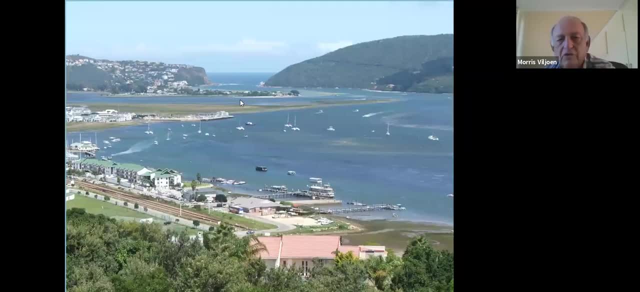 interestingly, in this place it's not a softer dune rock or whatever- that's where the mouth is, but it's actually very hard quartzite. a very significant band or zone or ridge of uh peninsula quartzite has been breached here by by the mouth of the niacin estuary. 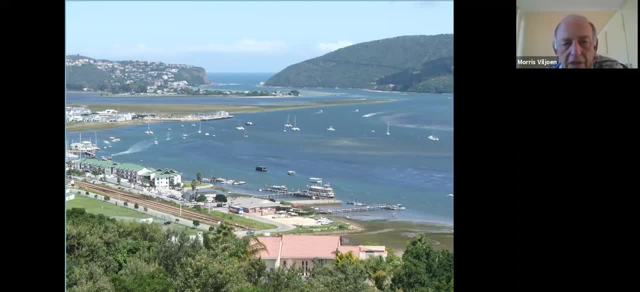 and the reason for that is that you've had incredible um structural uh deformation, faulting, fracturing, appreciation, and which has weakened the rocks in this area and resulted in the sea and the estuary being able to uh to bash their way through and make an exit for the niacin estuary. 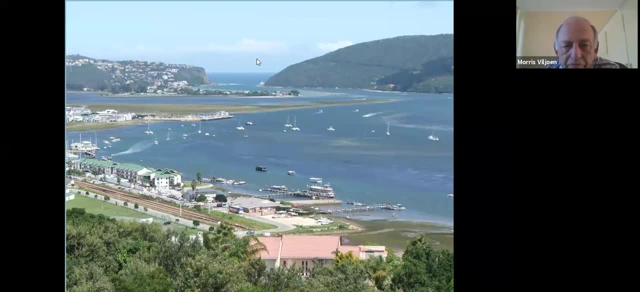 and that, of course, has been pretty significant. this niacin estuary has been a really important shipping area since quite earliest, earlier times, and ships used to come in here, through here, following the channel here, right up to the harbour- old harbour here- and a railway line came. 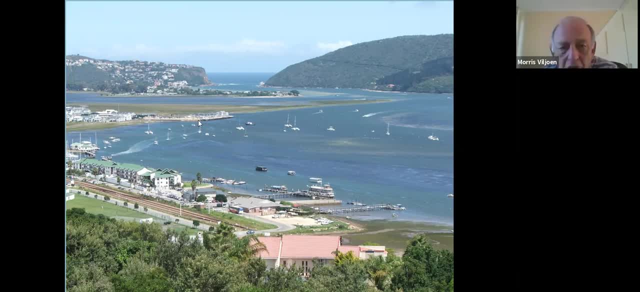 down the old railway tracks are still to be seen here on the harbour- and they essentially brought wood down. it was a lot of natural wood from the forests, of niacin, etc, etc. and niacin developed the wood industry- is what really developed niacin- all aspects of manufacturing and other uses. 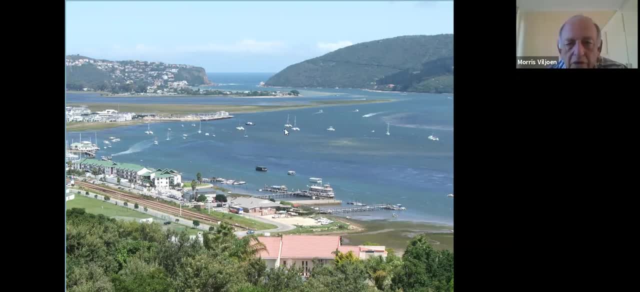 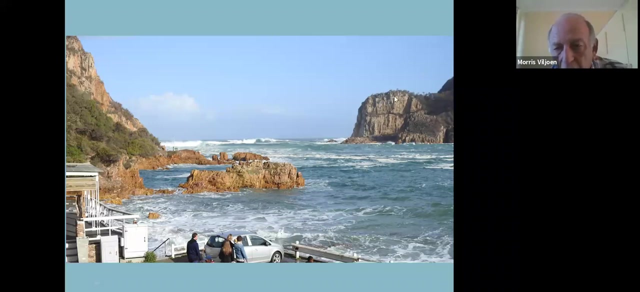 but a lot was also exported from here to other places and this is where it was loaded onto the ships. so we look now at how the mouth of the niacin estuary came about, and immediately when you get to the mouth you can see this: an incredible vertical verticality to the 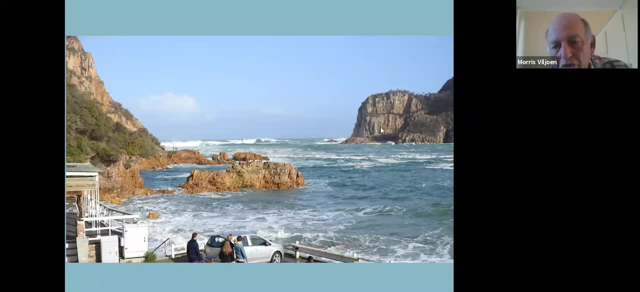 structure. these are vertical fractures and faults and whatever here as well. so the rocks are highly fractured, broken up by vertical movements, and this then became a weak zone where the sea eventually got through to form the heads and the here you can um, at cuba, you can get an an indication of how what happened. you can. 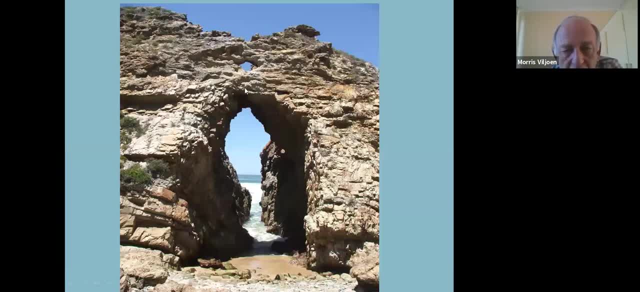 see a weak, fractured fault zone with breccia here and that's very clearly been preferential to the mouth of the niacin estuary. seeing how the the is this uh, this was the uh area that uh as the the major incisions uh into the. 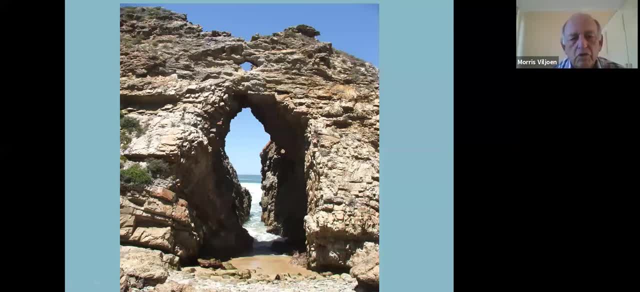 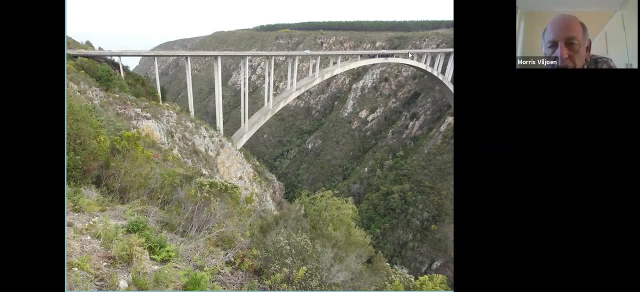 coastal plane along the tsitsikama coastline. so you're the part of the and the, such as Storms River and the Blowcrowns over here, which, incidentally, is the world's highest bungee jump. I think it's about 240 meters from here to the actual jump. 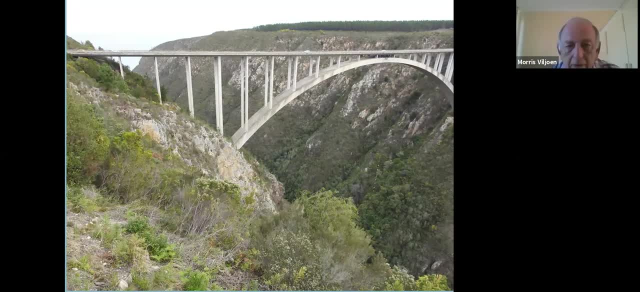 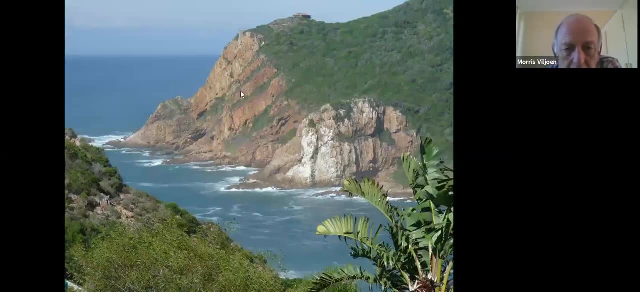 height of the bungee. Here you can see then a closer look at the Knysna heads, with the seaward dipping starter of the peninsula very regular there, with caves forming in slightly less resistant zones- old sea caves when the sea was at a higher level. 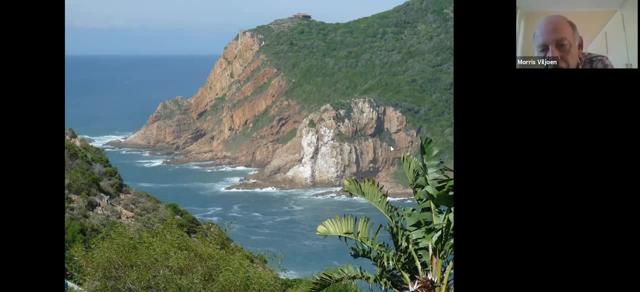 But then just look at this over here, these vertical shear fault zones that is preserved in this little block here But that would have obviously occupied the whole area and was preferentially eroded away. So that's just a remnant of what was there. 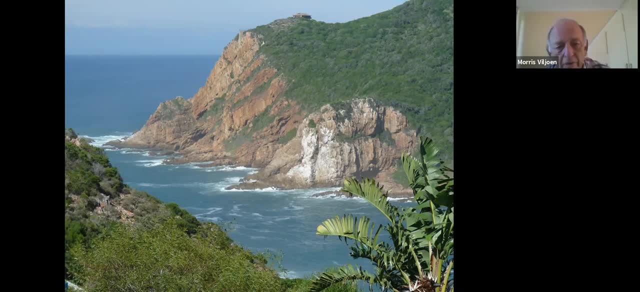 and what was preferentially eroded by to form this quite narrow gap of the heads. It's one of the most dangerous harbor entrances anyway, I think, And here's another example where you can see the process: the vertical fracturing and faulting. 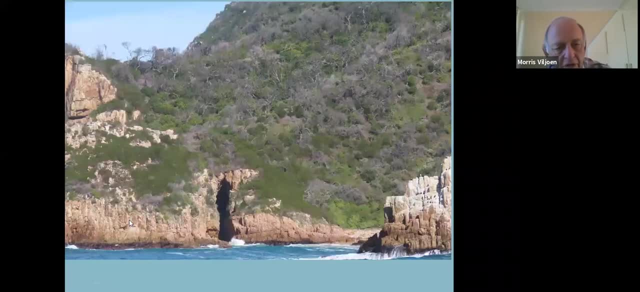 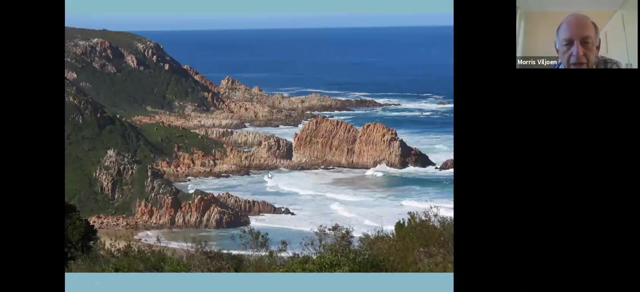 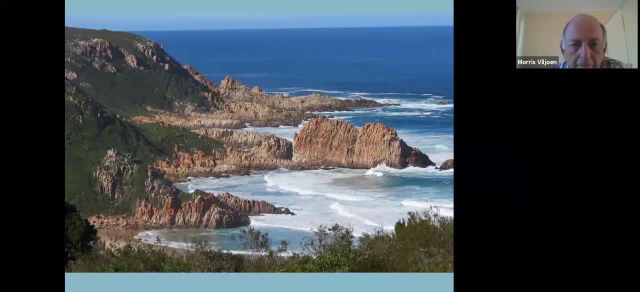 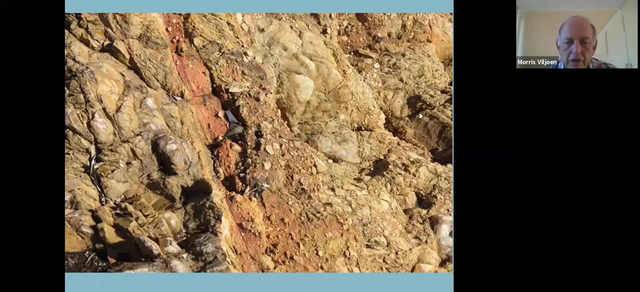 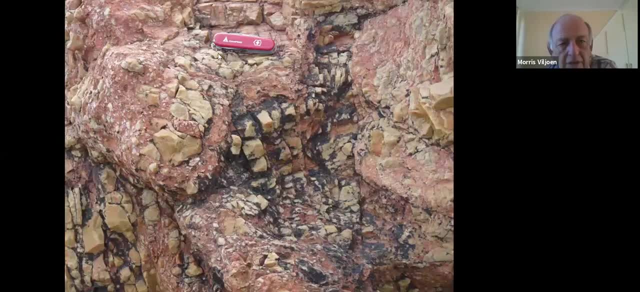 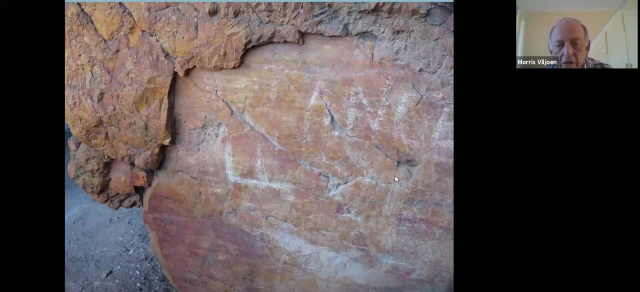 And what we have here is a precise example of high. These lines The normal. see these slickensides over here, horizontal slickensides. It's also become a popular spot for graffiti, but in any event, you can still see the slickensides on this flat surface. 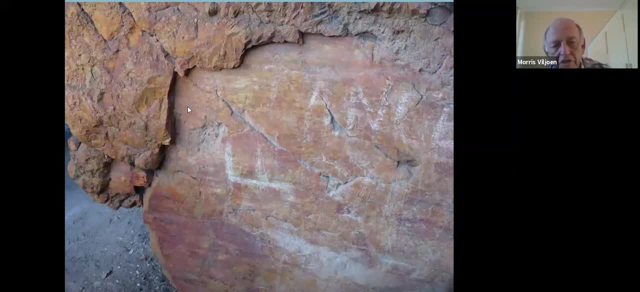 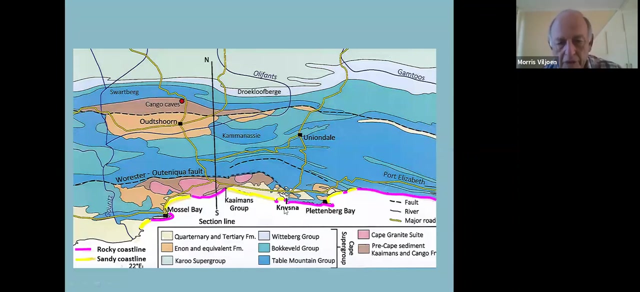 where the rock fragments over here scoured the surface and smoothed the surface and created these striations as well, A classical slickensided surface. Okay, and then the other thing then I have alluded to this are the coastal features, and you essentially get rocky coastlines. I'll mention those, Knysna heads here being one. 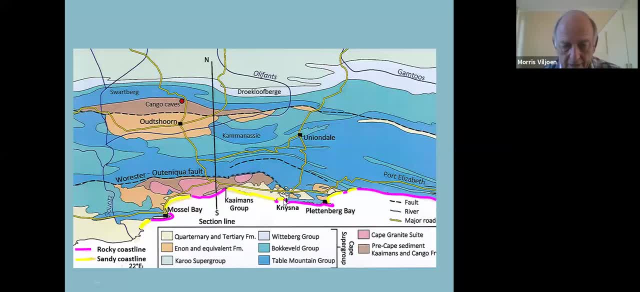 just a little rocky area due to hard rock And the whole of this Knysna Pletsch section, hard rock. This is a hard rock section, Mussel Bay, And then you get, and I mentioned a series of points, And behind the points you very, very very. 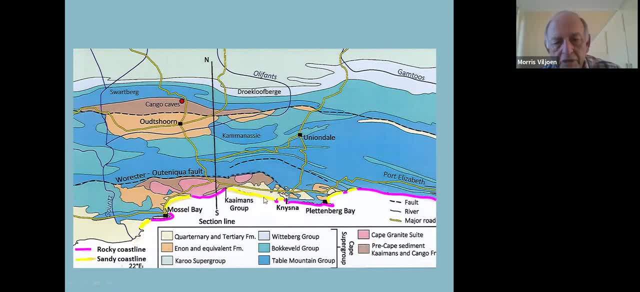 often you get softer formations. This is Enon and Younger. This is the wilderness embayment and this is Plettenberg Bay. The waves have deflected around these hard points and they've eroded into the softer material behind- That's the Mussel Bay, Plettenberg Bay, to form these. 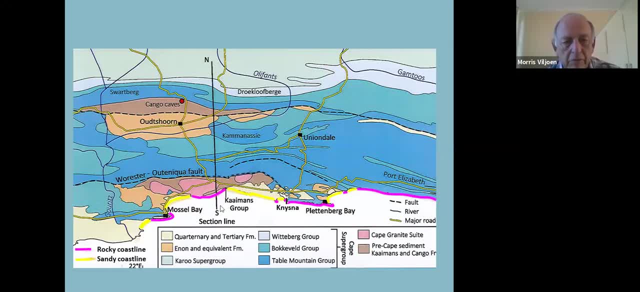 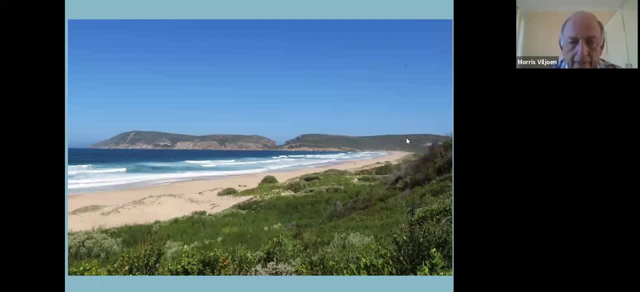 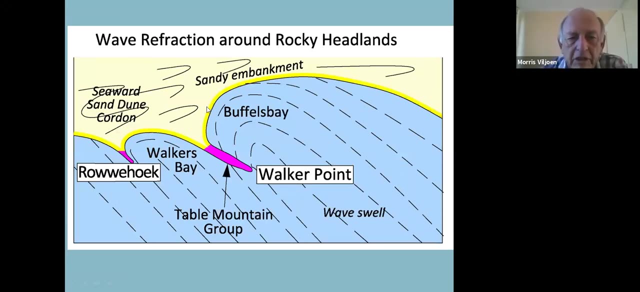 embayments, And there, for example, is the Rohrberg Peninsula and Plettenberg embayment coming around here, Nice sandy beach, Okay, And this is Biffle Bay and Walker Bay. We have a classical embayment, Biffle's Bay. 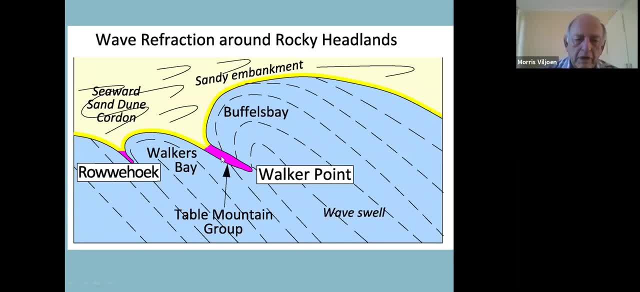 That's a very popular holiday spot, Biffle's Bay, and caused by this resistant walker point of quartzite. And then that extends away, And then another resistant quartzite pinnacle here called Rohrberg Hook, giving rise to Walker's Bay. So there's Biffle's Bay and 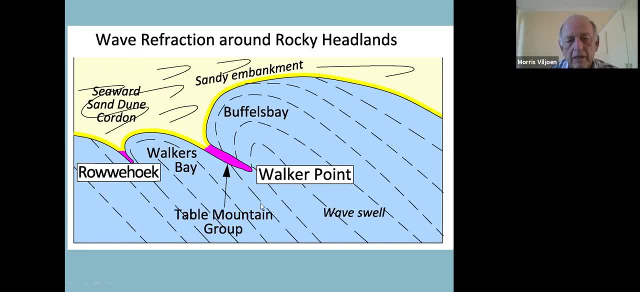 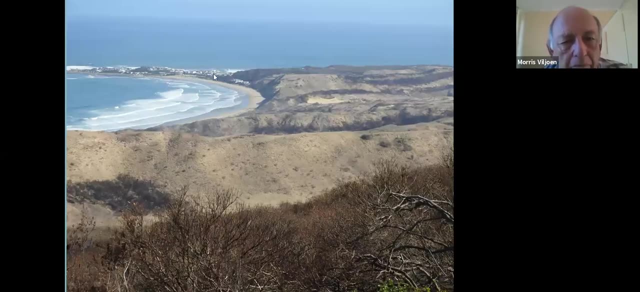 then Walker's Bay, So, and with the waves coming in, And the waves are coming in, refracting around the points and then coming in and eroding the softer material behind. So here is Biffle's Bay with Walker point resistant quartzite waves refracted around. 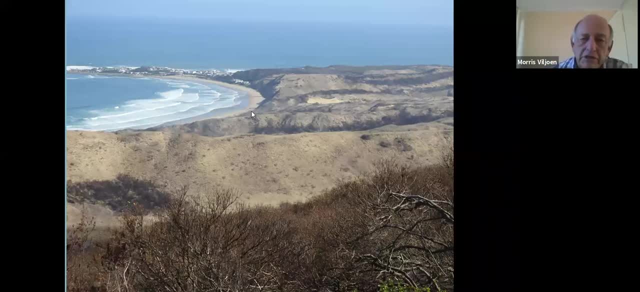 and eroding into the seawood dune courtyard. These dunes are pretty well, more or less as they were when they formed, Very virtually deflated, Very, very, very, very, very, very. no soil is developed, i should say, except along the base of the dunes, where you see some quite 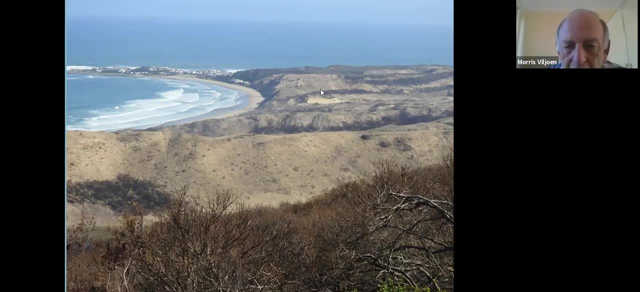 nice vegetation due to the fine material accumulation, nutrient and whatever, um, but this picture was taken after a major fire um two years ago which wiped out a lot of that vegetation. uh, it's come back again, of course, so what it normally looks like. so, but that gives to the 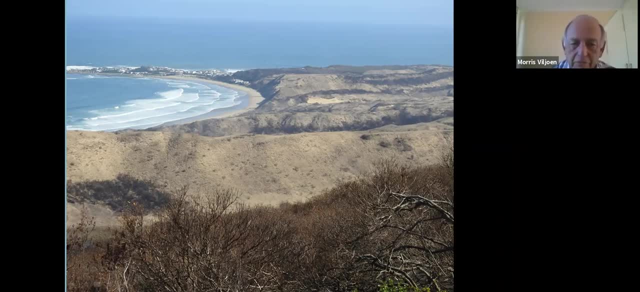 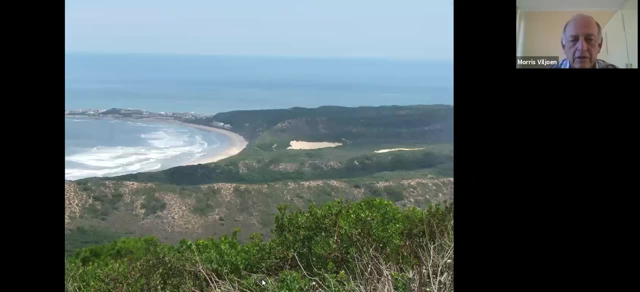 very sandy and dunes here with that much soil. that's what it looks like, now covered with a scrubby coastal vegetation, but you can still see evidence of these sand, sand dunes peeping through um. so, in any event, and that's an example, a classic example of a, of a 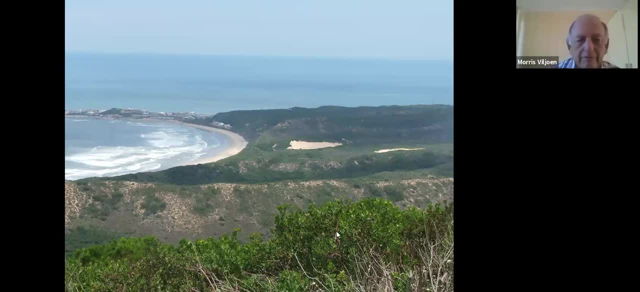 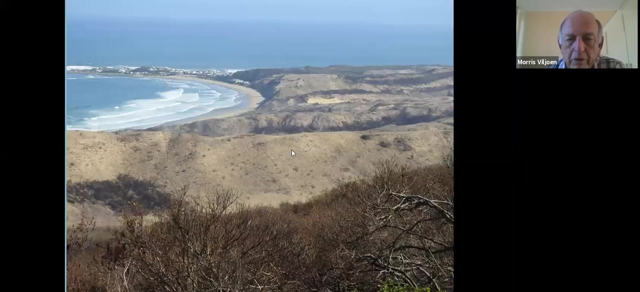 pinnacle, a peninsula or point, and the uh, the, the, the uh basin or the um sediment falls behind them. okay, oh, sorry. so there is in fact um, the walker, part of walker point, and then there's walker bay and that's rubber hook over there, another court side sticking out there. 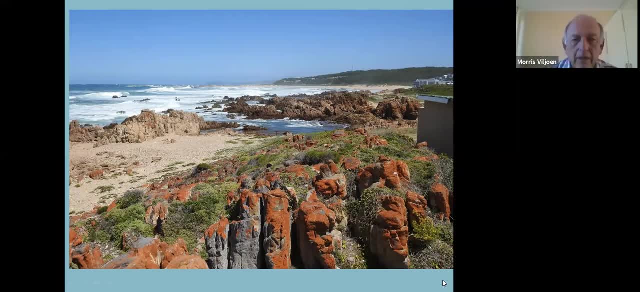 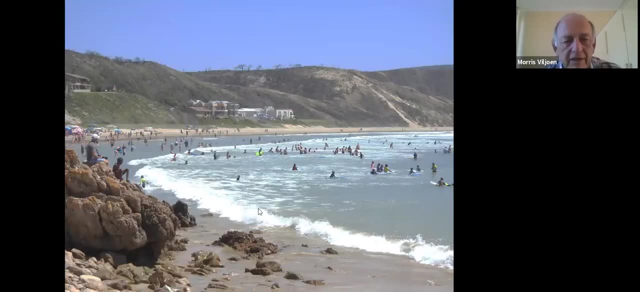 there's a walker bay around there, okay, and um, this is buffles bay, a very popular hurled a place, and here you can see clearly the resistant quartzite pinnacle point and then the less resistant material that's been eroded into to form this beautiful. 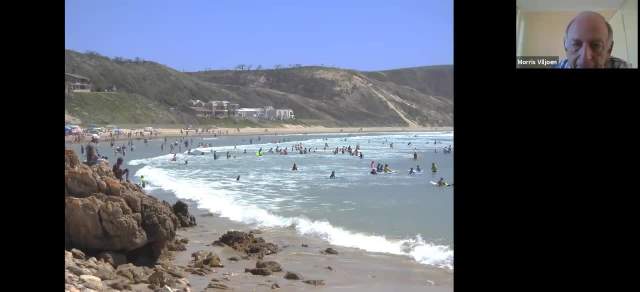 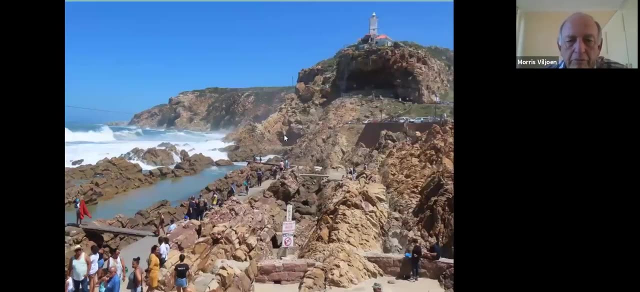 sandy embayment of Biffles Bay And another feature. another point is Mossel Bay Point, which is called Capes and Blaze, well-known lighthouse over here, And it is overlaid by younger this steeply seaward-dipping rocks which have been eroded. 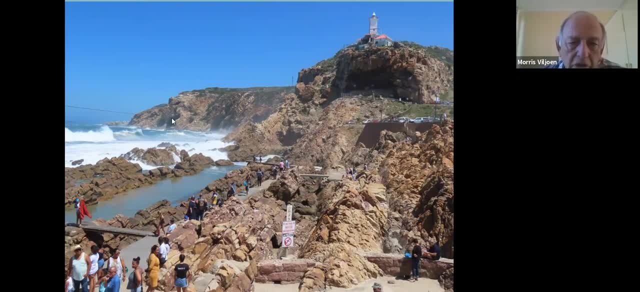 here You can see, preferentially by weaker zones, by different seas, and the sea was at a higher level And it's overlaid by younger, much younger, flat-lying strata of probably enon type. Nice cave here Capes and Blaze with some paintings and other artifacts over here. 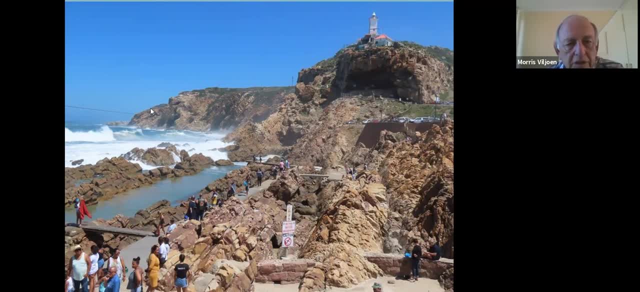 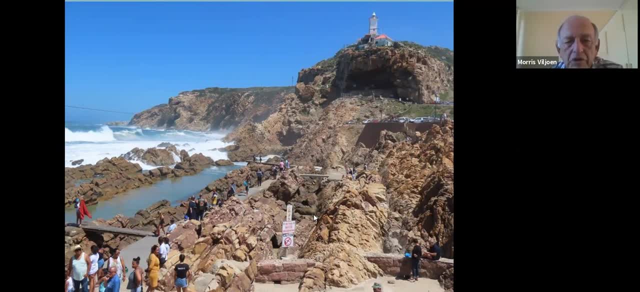 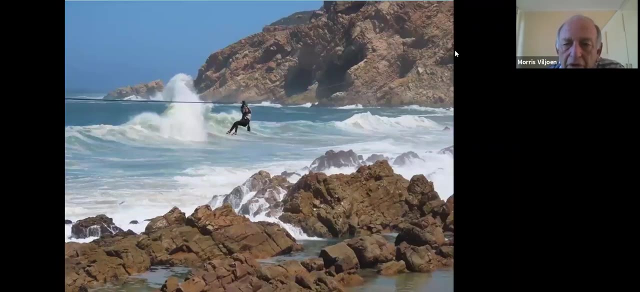 over here somewhere. It's a distance of 1.5 kilometers. It's the longest zipline over the ocean anywhere. And here we have the zipline in action and some of these preferentially eroded areas of the seaward-dipping quartzites. 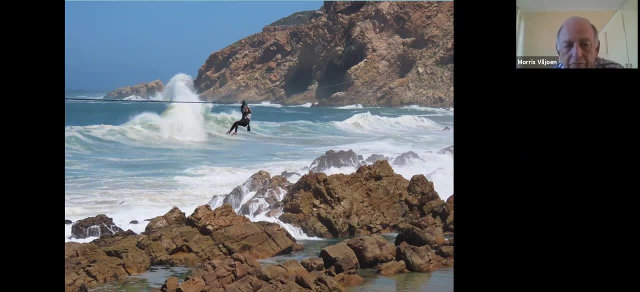 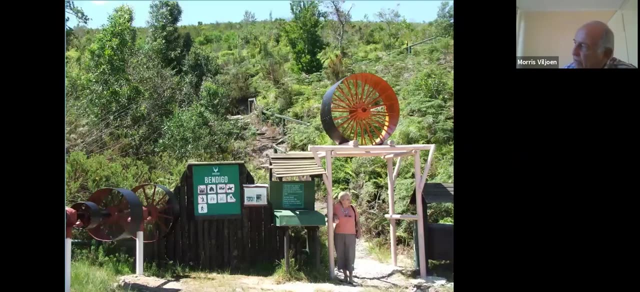 And then the other thing, And then the other thing, And then the other thing Of interest is the Millwood Mine gold mine discovered in 1880. About 1885, I think it was around about the time of the Wits discovery or just before. 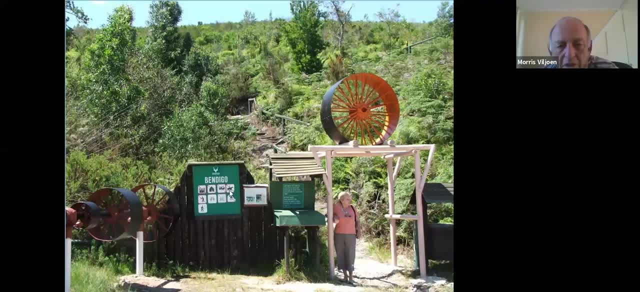 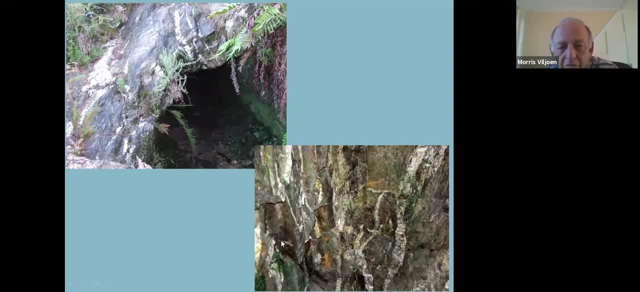 I think. But it only lasted a few years, but of course it didn't amount to much. Some of the old workings and some of the quartz veins are to be seen- gold-bearing quartz veins. There wasn't too much gold in them, I guess. 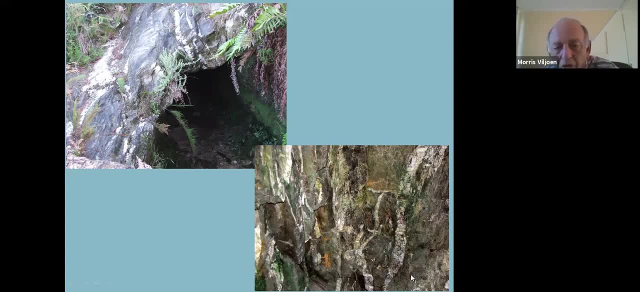 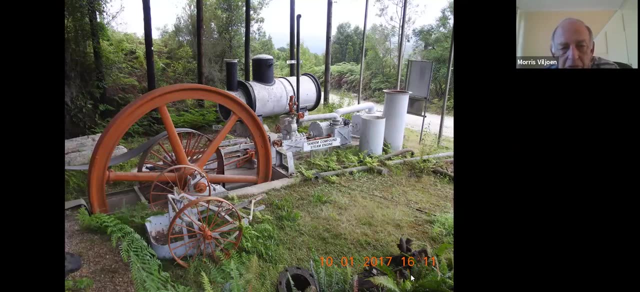 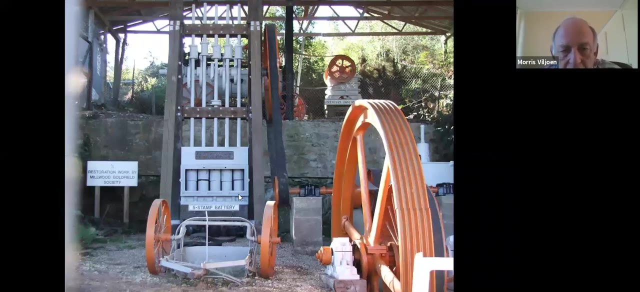 But. But they preserved some of the old mining equipment and so on that was used at the time. They'll stamp batteries and so on. So there's quite a bit of interesting historical stuff being preserved here, including the cemetery with a number of gravestones dated 1889.. 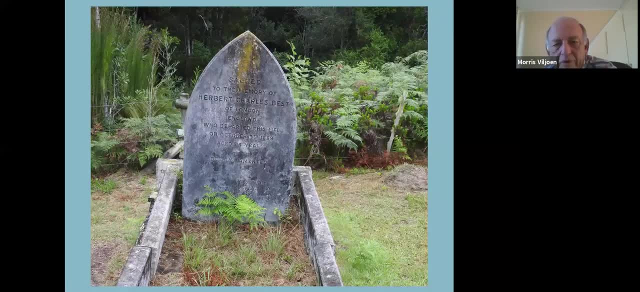 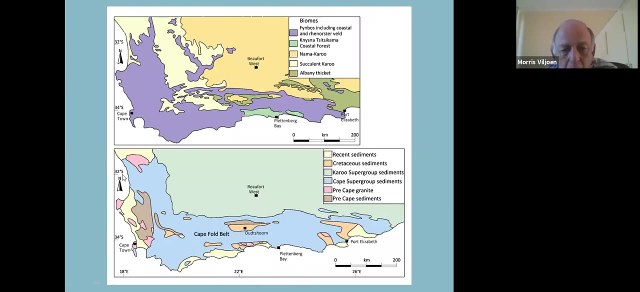 Yeah, that's about the time also that it started packing up because it wasn't lasting and the Badwadisrant had taken it off. And just to get on to the floral story, this shows the Cape Quartz sites and Fold Mountain distribution, with the underlying caimans and granites, the Cape Granite here and the 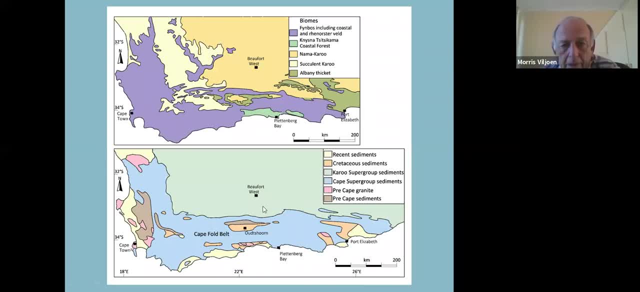 Mahomes Bree, etc. the older stuff. But then this is the distribution of the Fanebos biome, which are very unique in many ways, And it also includes this biome here, the Knysen at Tsitsikama Coastal Forest. 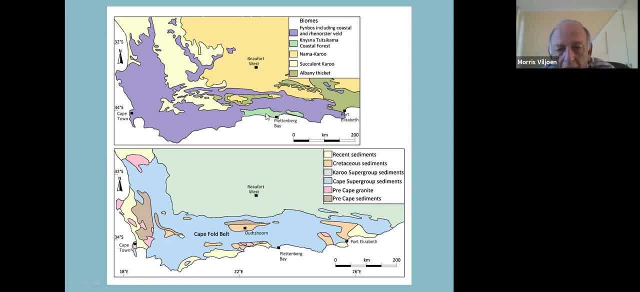 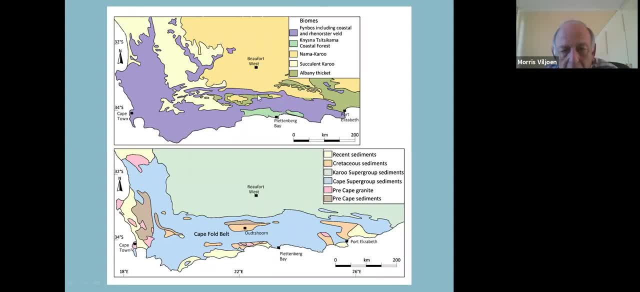 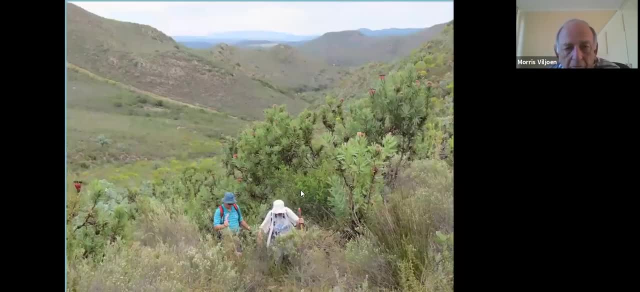 So this is the Fanebos biome of this southern area over here. This is a typical Fanebos type: covered hills and mountains. you find Protea being pretty evident, But there are other types such as these Erechons and Restiers. 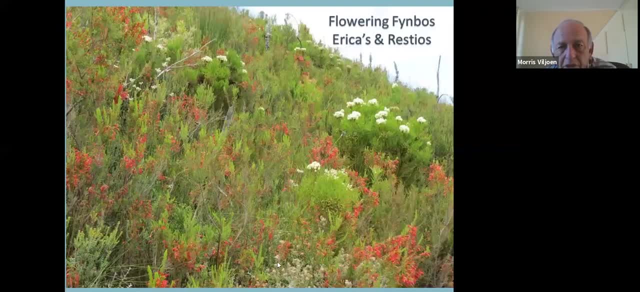 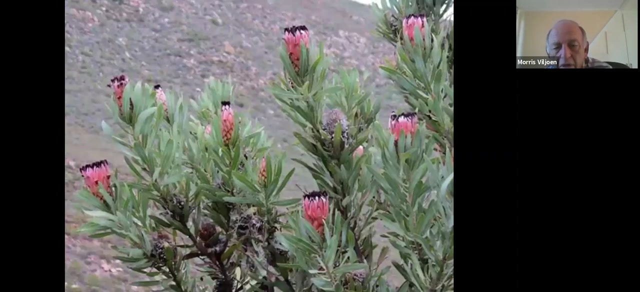 Restiers. I think it should be an A, But very attractive and very distinctive Fanebos types are very prevalent, And then, of course, proteas, our national flower, and then these forested areas still preserved in some of the valleys, in some areas, these classical coastal southern afro temperate. 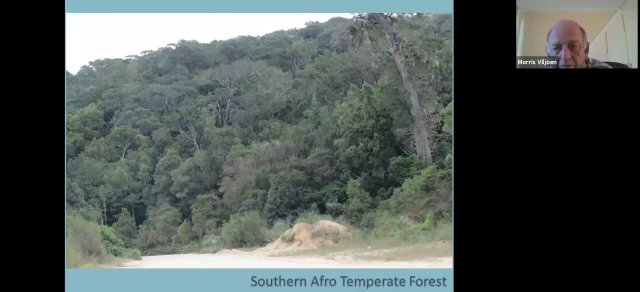 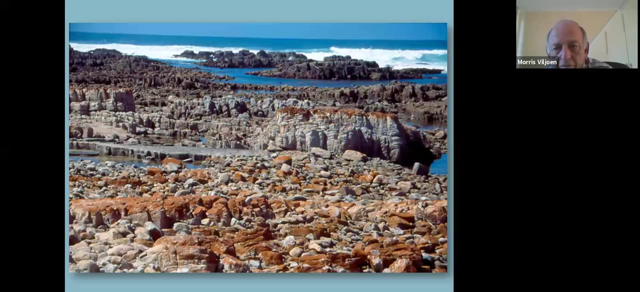 forest it's called. And then just a bit on the human history. once again, everything controlled by the underlying geology. and here we have flat lying strata of hard quartzites, but flat lying, but also with strong vertical jointing in this case, and there's an old wave cut platform and it's 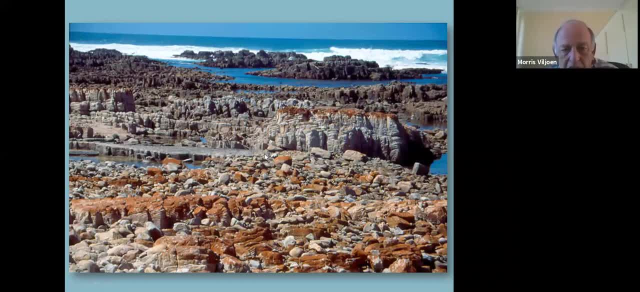 broken up the rock because it was nicely fractured and jointed etc. to form big chunks of rock which were washed around on the coastal plain over here and became rounded boulders And the old timers, essentially the Koi people, started gathering this rock and building. 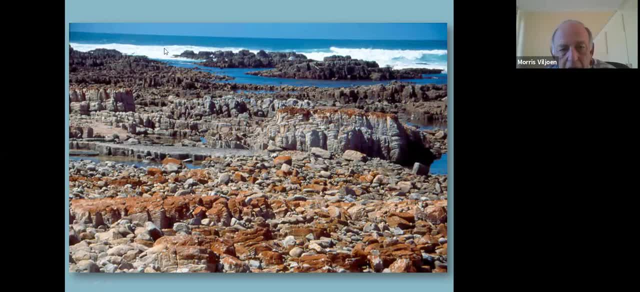 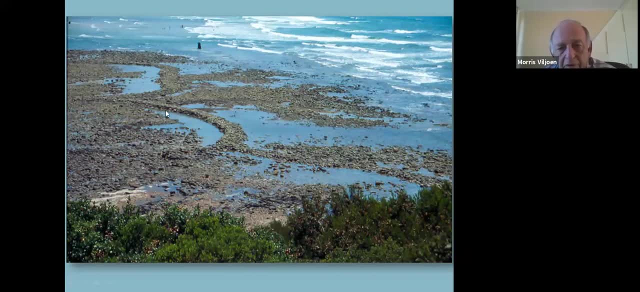 what are called fish traps over here steep inner side and a gradual outer side. so tides came in, brought the fish in, and when they went out, the fish were trapped over here, And so- and there's some really good paintings- this, I think, is quite a classic- showing the 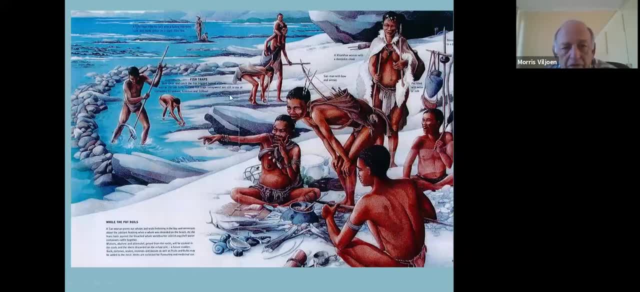 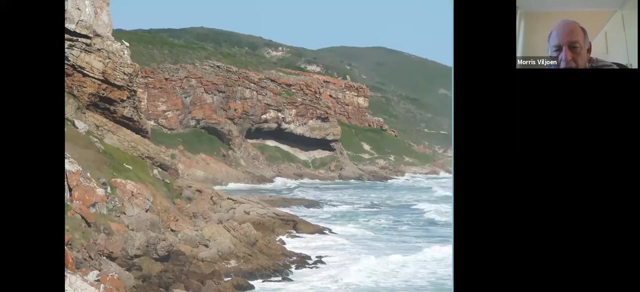 activity in the fish trap, Eating the fish and coming ashore and eating the seafood over here, the early Koi people. Okay, here we have the one of the classical caves, and many of them, that occur in the coastal area. This is on the peninsula and in fact there are about a dozen of these caves on Rhôvôr. 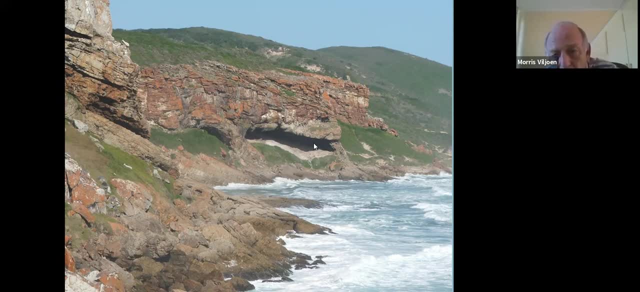 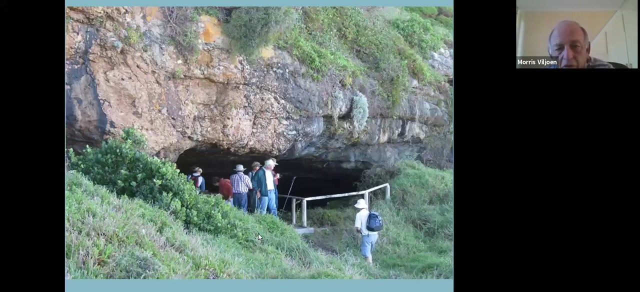 Peninsula And most of them have some form of midden. there's accumulation At the base with signs of early human activity. This is a cave called Nelson's Cave. This is on an archaeological tour of the area I did a few years back. 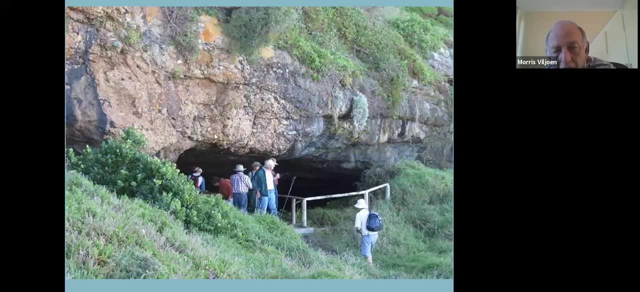 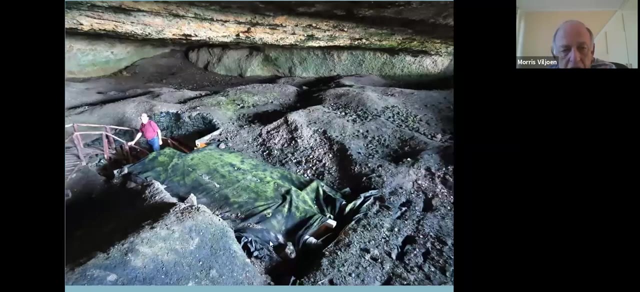 And this cave occurs at the base of the Enon-type conglomerates and the underlying peninsula quartzites. It's quite a spectacular cave and a very significant deposit, and a lot of excavations have been done. This is the main excavation site over here. 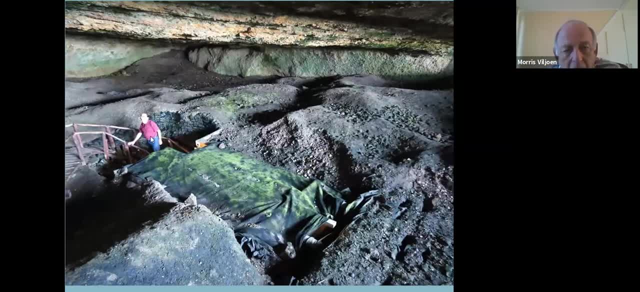 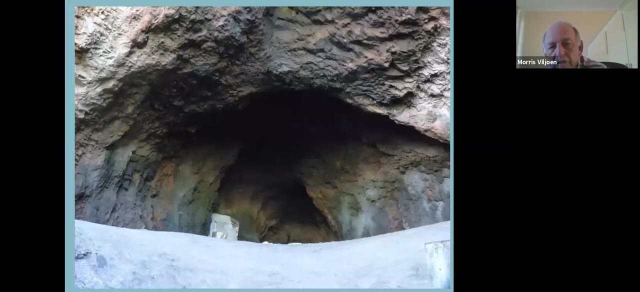 That's a guy called Reinhold Buers. he was the leader of this trip. he's quite a big figure in the archaeological society. And so there's the Nelson's Cave, and then the other one is a cave on the east flank of the Knysna estuary. 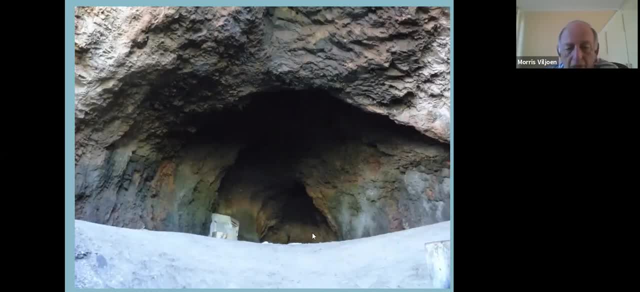 And you can clearly see here how a fracture once again, but now this is an east west trending fracture, not typical north south east west trending fracture fault zone along here which has been preferentially weathered in an east west direction. now, however, 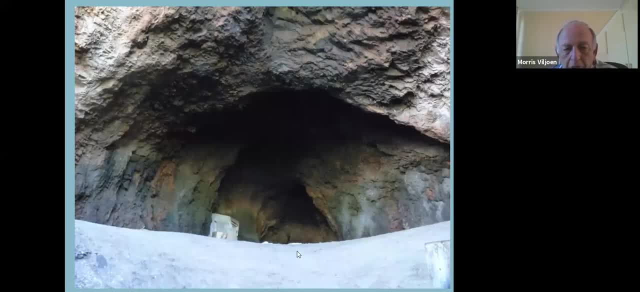 And what you see in the foreground is a midden, a pretty significant midden, And that midden was excavated by Thomas Bain in about 18, I think it was in the mid 1880s in fact- And when he was building the roads, when he did the famous road builder and his father 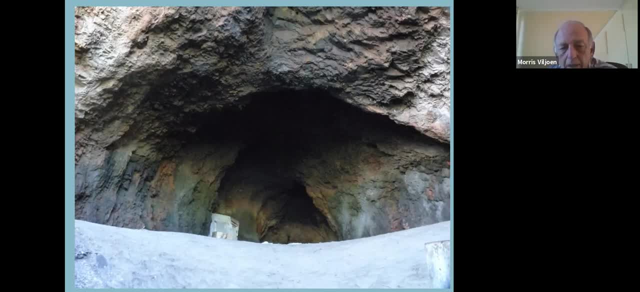 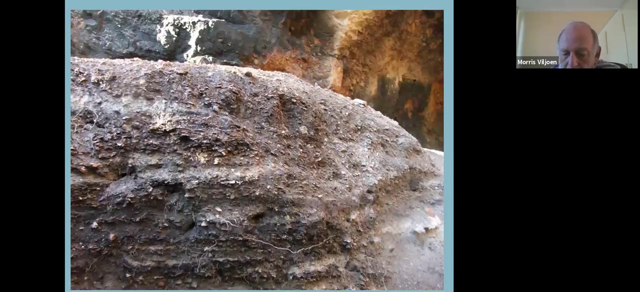 was Andrew Geddes Bain. Thomas Bain was the son. this is Thomas Bain, then, who excavated here and, amongst other things- and that's the typical midden in the cave of shale, fragments and all sorts of archaeological artefacts have been found there as well and, incidentally, 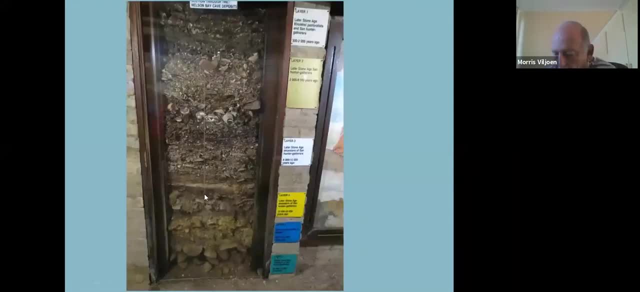 from a study of the deposits in the cave, you can actually see episodes where the coast was close by and you can see a lot of seashells, and then other episodes when, which are kind of devoid of seashells, and those can be areas when the sea level had sunk and that the actual 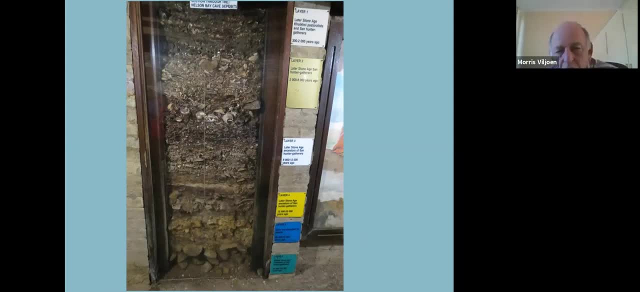 coastline was quite a long way away. So it's all documented here. they give the ages from about 12,000, greater than 12,000, here 8,000 to 12,000,, yes, 12,000 to 8,000, 2,000 to 8,000, etc. and then 2,000 to 300,. 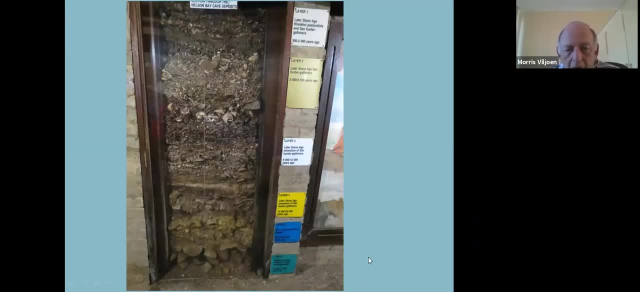 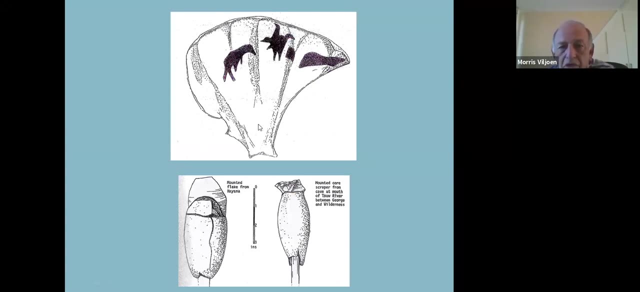 etc. So it's pretty been well documented by archaeological studies. Amongst other things, Thomas Bain found this here, which in fact it turns out to be the scapula of a seal, And on it we can see a little bit of the shape of the shell. 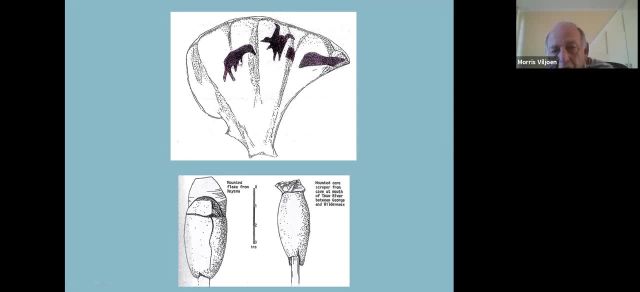 And on it we can see the shape of the shell And on it we can see the shape of the shell. So they were paintings, or half. they found paintings of what appear to be possibly a seal, a bird and a whale, and also under artifacts like these flints, flakes melted. 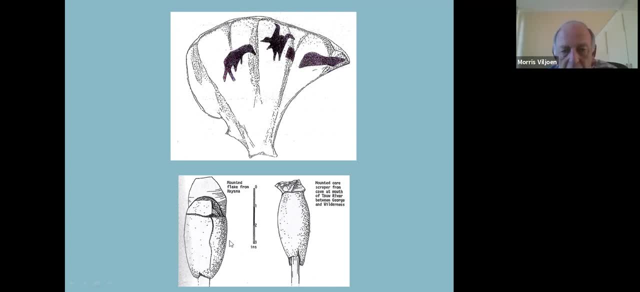 on like this over here for scrapers and whatever. And that artifact there that is called was taken to an exhibit in London in 1886, in fact, and on the way back to South Africa disappeared, But then miraculously, somebody then came to the British Museum and sold it to them for a nice price. 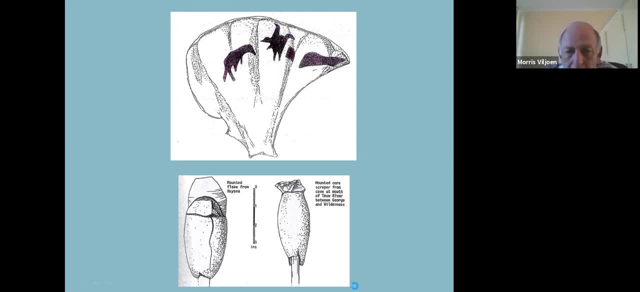 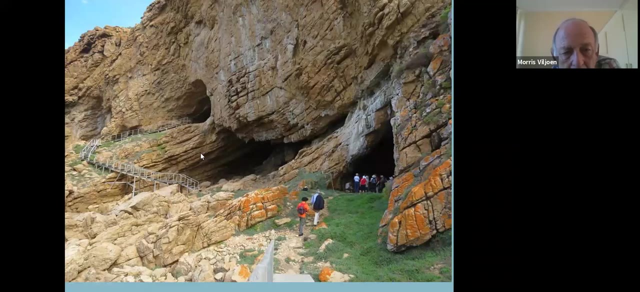 and there you can still see it Right. we have some more interesting cave areas. This is the Pinnacle Point Cave. Once again, a number of cave systems have kind of formed and some actually coalesce, And it's in here that some of the earliest forms of human-like activity 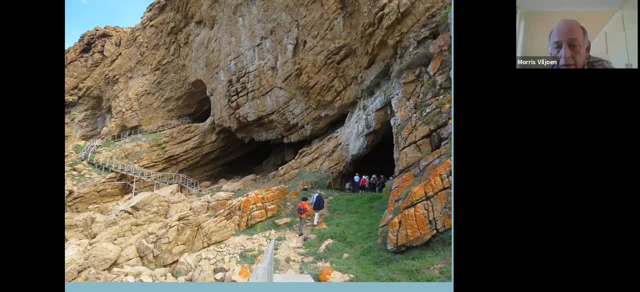 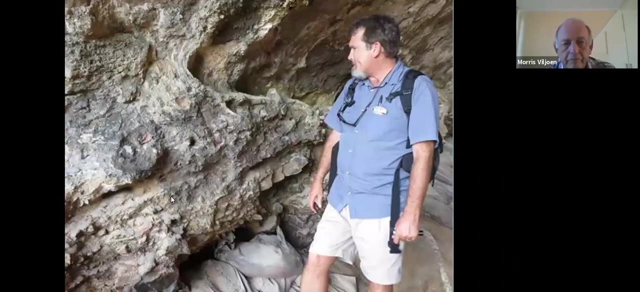 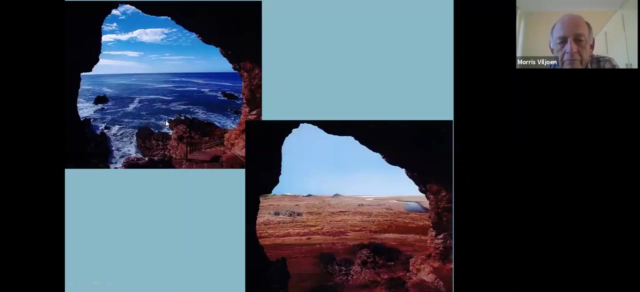 the earliest known actually anywhere of human-like activity have been found at Pinnacle Point, And here are some of the breccia found in Pinnacle Point And when it was inhabited. at that time, 160,000 years ago, the sea level was way up. 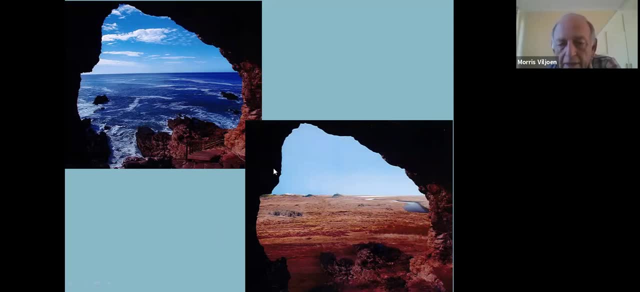 and you can see the coastal dune field in the distance and you can actually see the coastal plain exposed And these guys were foraging here for food and there was some animal life as well, doing some hunting and bringing the material back to the cave. 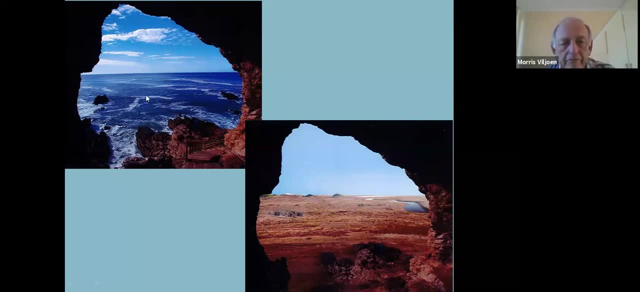 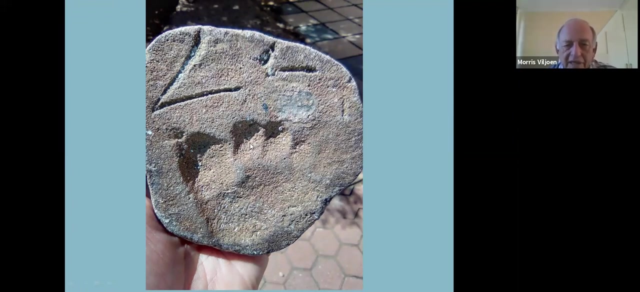 And that's what's preserved now at Pinnacle Point. That's what it looks like now, That's what it looks like today. And in that area, Belinda down here, a coastal lady who's into collecting stuff, found this: what seems to be the footprint of a child's footprint in calcified dune rock. so from about that era. 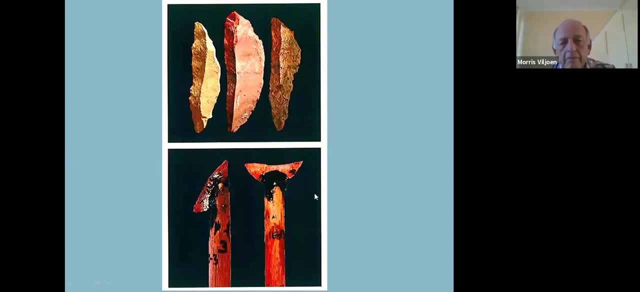 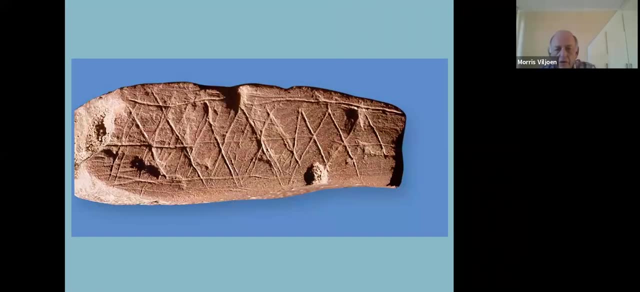 And also these flints have been found as well, and various cutting-type tools, by the looks of it. And then there's also quite a famous artifact, and it's essentially from the Stillbay area. It's actually a piece of ochre with a chevron pattern carved onto it. 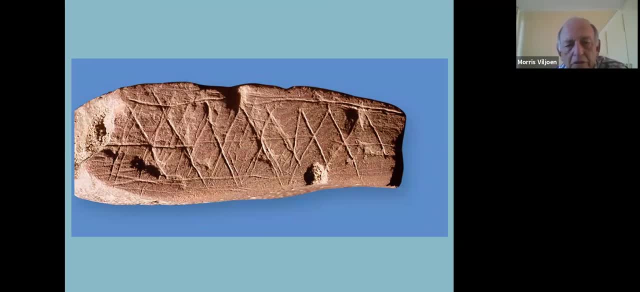 and that is considered to be human-like activity. I mean, chimpanzees are pretty clever and they could probably cut a piece of rock like that, but it's unlikely they'd sit down and deliberately create a chevron pattern. But it's unlikely they'd sit down and deliberately create a chevron pattern. 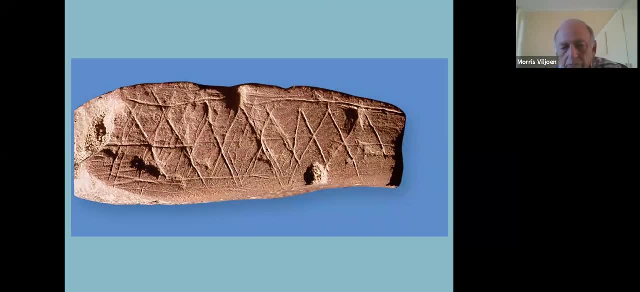 That is considered to be human-like activity, and it is in fact the first evidence of human-like activity. This, I think, is dated at 80,000 years, And then here's a painting by Maggie Newman which sums up the whole situation at about that time. 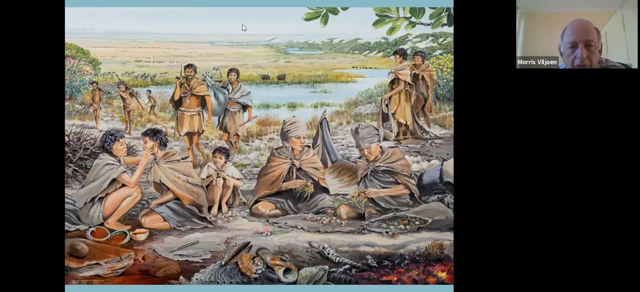 Early people, earliest humans, gathering plant material as well as hunting, bringing in some animals that they've killed. And then people have collected seashells over here, and then others are using ochre to decorate themselves, and you can actually see the chevron pattern of that little artifact. 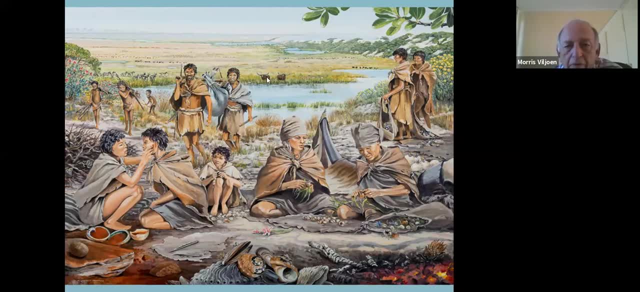 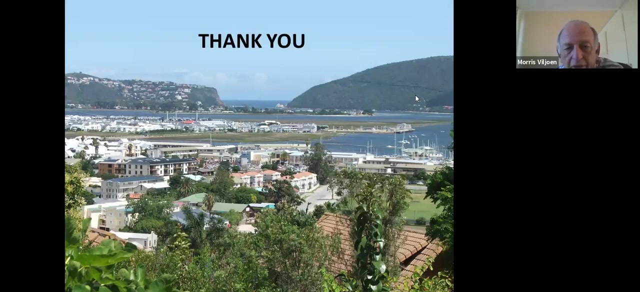 And some of the long-horned buffalo extinct, and that is the coastal dune. at the time that this was taking place, This would have been about maybe 140,000 years ago. So that is a brief review of the geoheritage of the Southern Garden Route area. 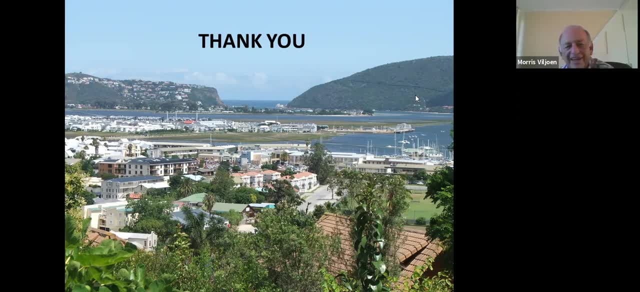 And thank you very much for listening. Thank you very much, Morris. That was a very well-illustrated talk. I'll open the floor now for questions and comments. So either raise your hand or just unmute yourself and go for it. 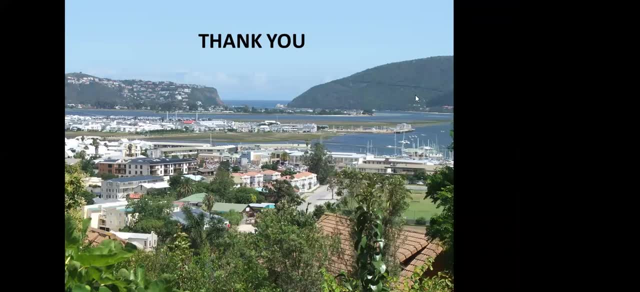 I'd like to start the commentary with just a question. I mean, is there in existence any sort of publication that makes the geology, the geomorphology, the botany, the archaeology and the anthropology available to the average tourist? 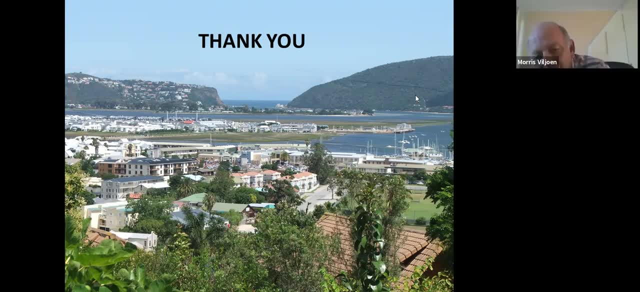 Is there something like that in existence Or is it being planned? Not really, but there will be one soon. I've actually written it and it's ready to go, And in fact, just about all the slides that I've shown you will appear in this booklet. 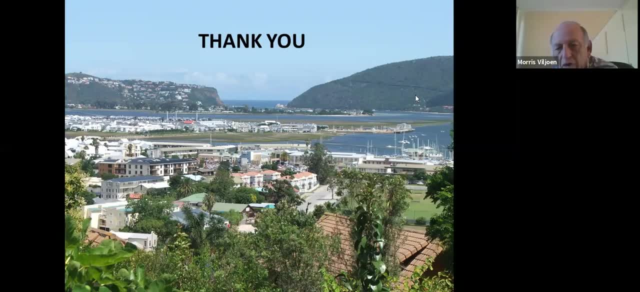 and a brief summary of the whole story, And I think I actually showed some of the sites that are included as well. It's a tour guide of the Garden Route and it essentially tells the story as I've told it basically, with the sites where you can actually see. 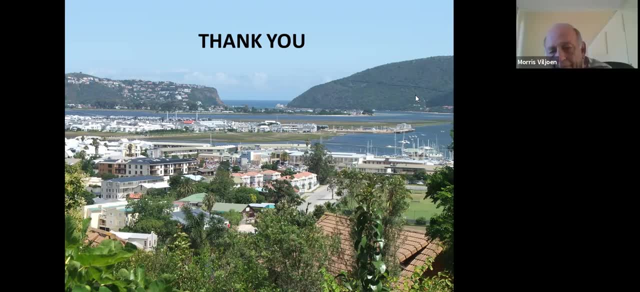 What is being talked about? Okay, Robert Smith has a question. In fact, maybe the Society would be interested in publishing it for me. I think we must talk about that. Okay, Robert Smith asks: can you comment on the cause of the recessions of the shoreline in the Miocene? 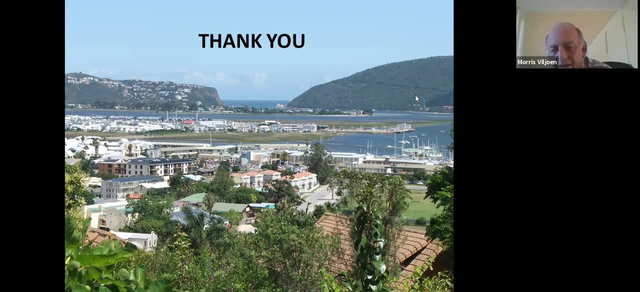 It was unlikely to be diesel engines. Yeah, The shoreline is generally considered to be a result of colder and warmer periods, When the ice cap froze up and froze the water from the water of the oceans. it was frozen in the ice cap, essentially, and resulting in sea level drop. 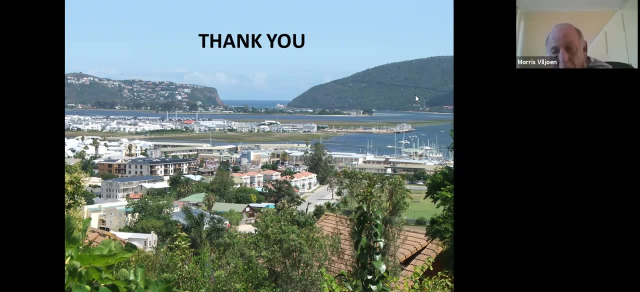 But there might have been some tectonic activity as well. I'm sure there was also, But essentially it seemed most people seem to think it's sea level changes are due to changes in temperature, And I showed that one graph which was essentially of temperature over time. 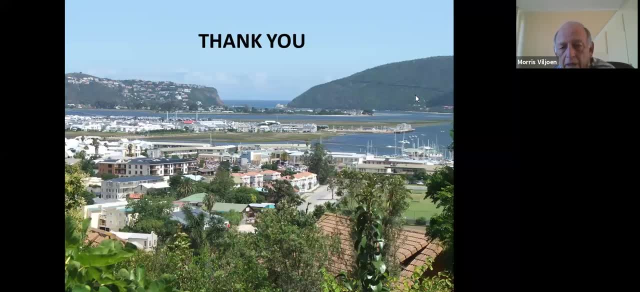 And that's how it's been worked out. So clearly, there were these major fluctuations in temperature. Now, what caused those, of course, is another story, which I'm not sure what the current thinking on that is. Okay, Thanks, Morris. 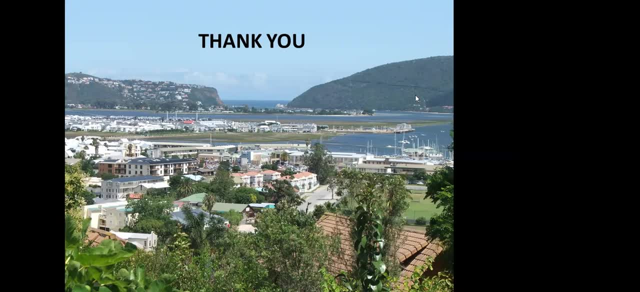 Any other comments or questions? Craig, this is John Bristow. Can I come in here? Yeah, Thanks for an interesting talk. First question, Morris: Those really nice cross-bedded young sediments along the Renton Cliffs, is that the low or your equivalent of the Bredaarsdorp stuff that we get down here on the Cape? 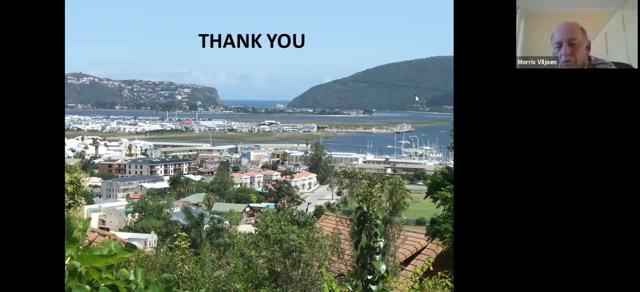 John, I should think it might well be, but I'm not too sure about that. I haven't really seen the Bredaarsdorp stuff. I haven't really seen the Bredaarsdorp ones, But it sounds from what I've heard about it it's quite similar here. 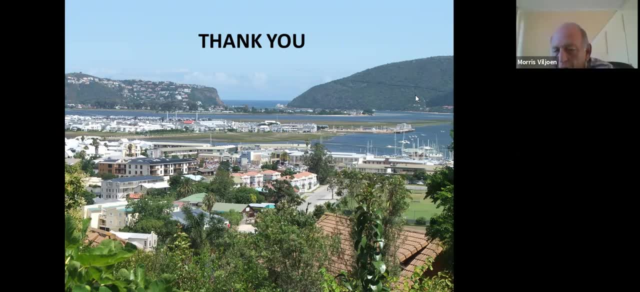 It would be the same thing. The same sort of processes would have operated right around the southern coastline, I think, Because I've certainly seen. you know these sorts of little features. On the Natal coast we also get classified dune rock at Umshlanga, I think it is. 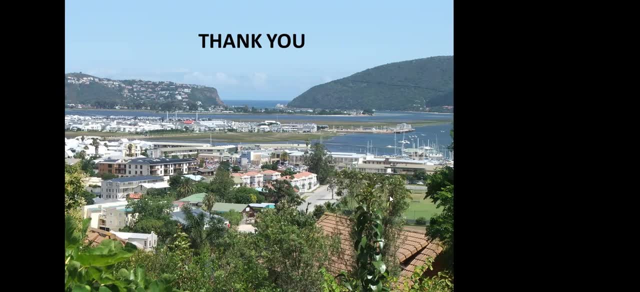 I remember seeing, But I haven't really studied any other area in any kind of detail. I've just had glimpses from time to time. So it would be interesting to get information on other areas and see how it compares to the story developed here. 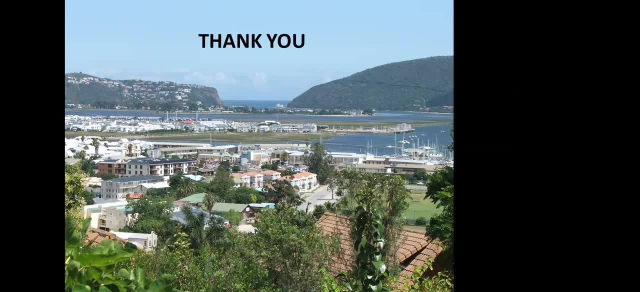 Okay, great. And then the other comment, and it's great, you got into, you know, the modern development of people in the Khoisan and all that, But there needs to be a hookup with people, With people like Hayley Korthra, who's an absolute wonderful resource and a young person. 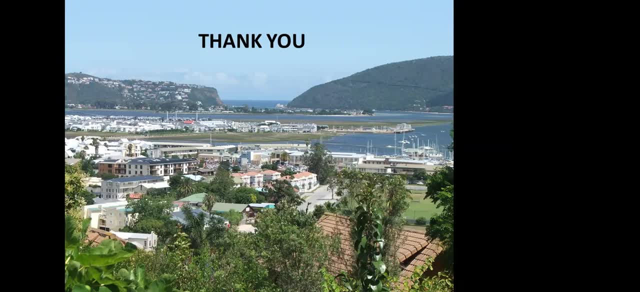 And unless we, you know, get involved with our young people, we're going to lose them. She's at the CGS in Cape Town And she's obviously it's been sort of slightly more orientated towards the Agalas Plateau and that area. 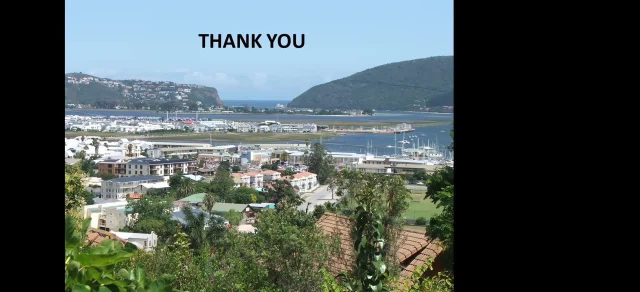 But she and others have done some amazing work on the very young you know- coastal geology, the climate change- I think it's part of a CGS climate change, The CGS climate change project. And, like you talk about the caves there down here, the caldars around the corner from Hermanus in the caldars are just world class. 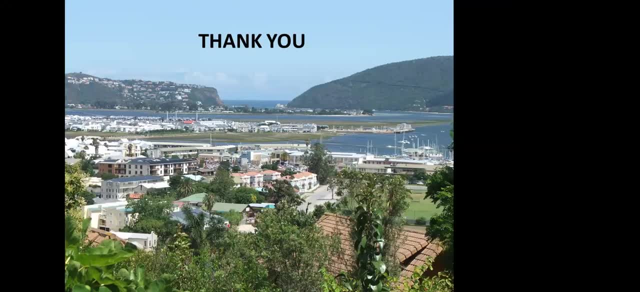 And the work done there by you know, the Eka Museum here in Cape Town and other people. it's just spectacular. So you know, in terms of fitting this together, you probably should spend some time with her. She's just a wonderful resource. 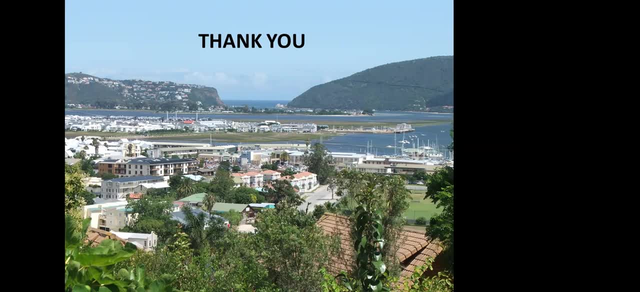 And she's also dived in a lot of these areas and you know, gone and taken your coastal on land work to the drowned beaches effectively. And then my last comment and last question, And it's to me it's probably the most critical of all of this. 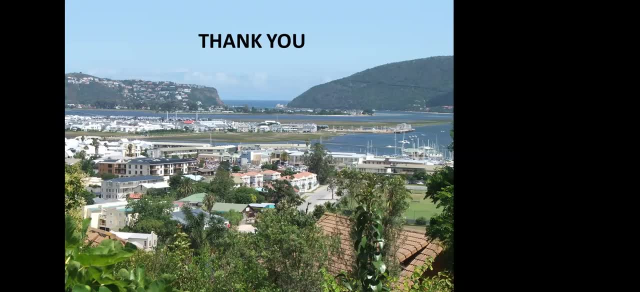 And I'm not looking to be critical, But all this geoheritage work, is that aimed at us geologists who are, you know, you're talking to the converted- Or are we looking to take geology to our communities and kids for the future? 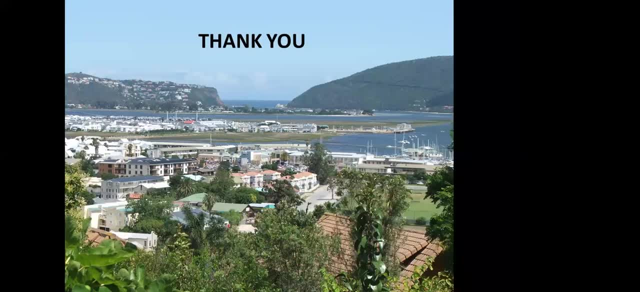 Because you know, that's my biggest concern. And then are we looking at places like Maconjuan and learning from that, Because there you know the work that's been done and the way the information is presented. it's presented for the layperson. 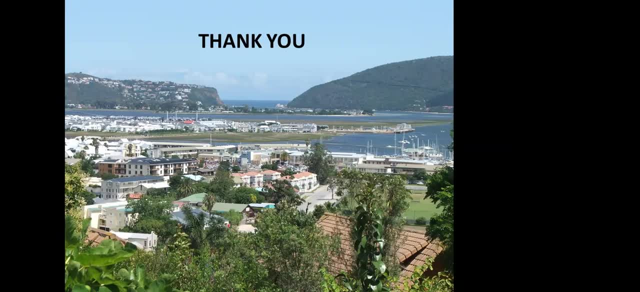 You know, and I listen to a talk like this today and it's fantastic, But it's very much it's a technocrats talk And I say that positively. But unless we start getting this amazing geology of ours down to kids and the people of the future in this country who are obviously not of our color, 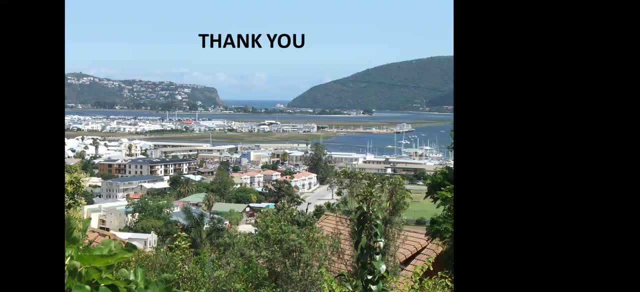 And the politicians. you know, our profession is on a hiding to nothing, sadly, And that's my, you know, sort of parting comment is: how do we take all of this amazing stuff that you know determines the soils? The soils drive our agriculture. 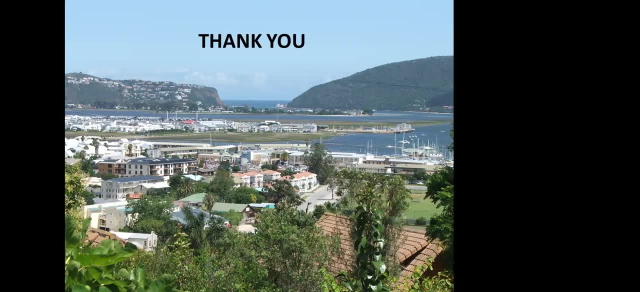 You talked about the Fane boss. You know how do we get to the people that really matter for the future, Because you and I are, you know, unfortunately a dying breed And if we really want to leave a legacy, how do we get you know down to the real people that count? 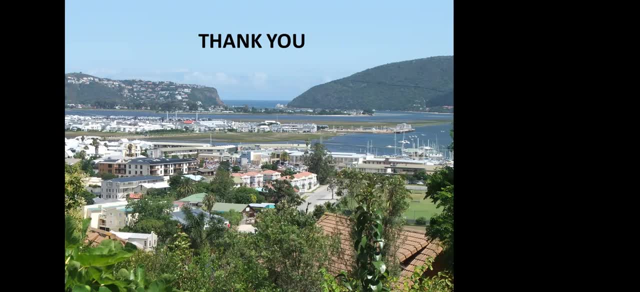 That's my comment. stroke question: That is also our big worry, John. Absolutely. It's very difficult. You come to the conclusion you've actually got to put this material across at three different levels. It's almost impossible to put it across in a way that's suitable for everyone. 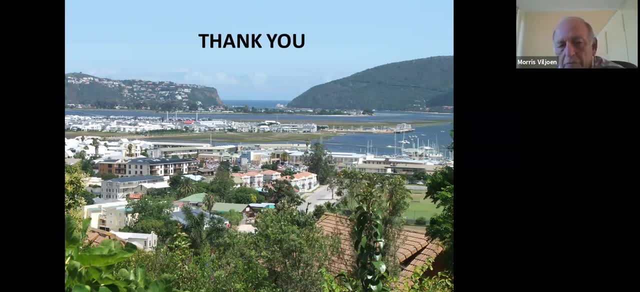 So you've got to decide at what level you're aiming this And this particular one is aimed at a relatively high level. but for the seriously interested traveler, I think you can't do it without the people who are the geological, geographical background and so on. 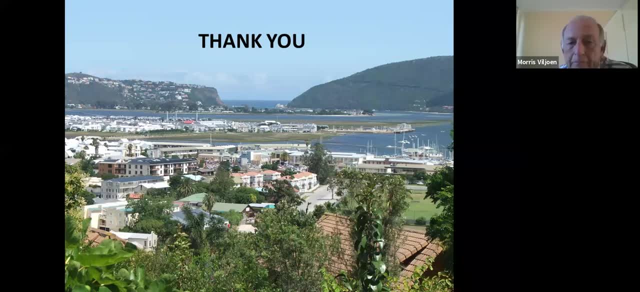 And I agree that needs to be dumbed down, if you like to call it that. And one has got to think hard about doing that. It's not easy, It can be done And we need people who can do that. And, Yeah, the key thing now, Morris, we've got the people we need to use, people like Dave Marant and that who sits down here in Betty's Bay. 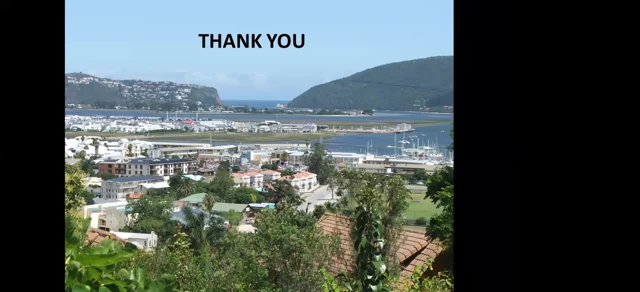 And was intimately involved in in Mokonjwa. So we have all these resources and we, you know, somehow- and I'm not talking group- think where we, you know we're going to end up doing the same thing as this. 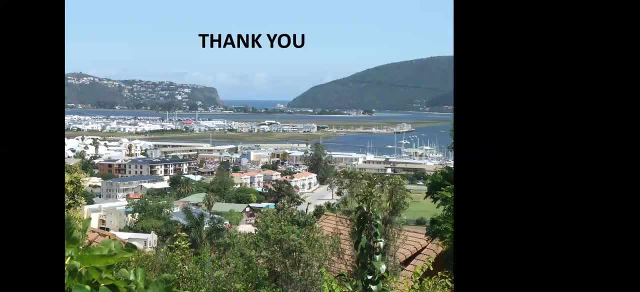 How do we start? you know, getting this stuff to, as I say, the people that count. I agree, It's a worry, really. How are we going to do this? But we need- I need- to work. We want to open this up to as many different people as possible. 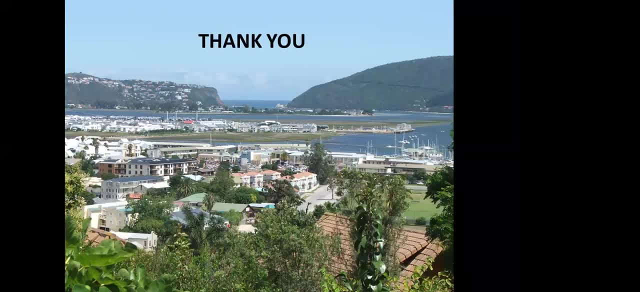 And and also up to the tourism industry. The tourism industry because you know, we think it is a potentially very good tourist product But, as you say, it's got to be put across in a more, much more simplistic way, And we need to work with people who can help do that. 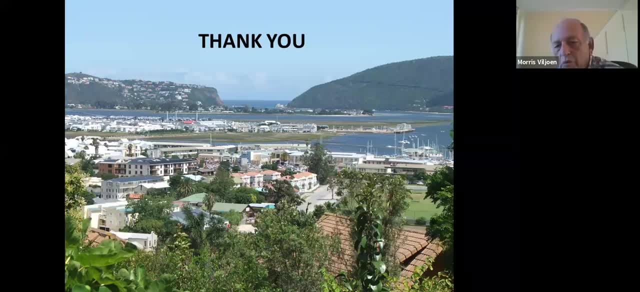 And so, yeah, I agree We need to. It's got to be done. I need to need to. I have had a chat to Hayley Cawthorne a little while back. I need to speak to her again. I'm going to have a chat. 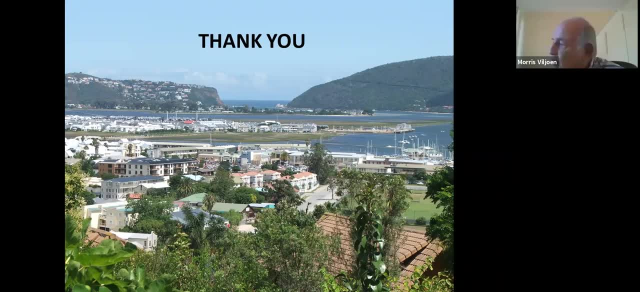 Sandparks operate here. They are out of wilderness, They offer, they've got a scientific office there And most of the area I've talked about, or much of it, is covered by both the and the, by a wilderness of national national parks and parks, as well as by the Hukama Nature Reserve. 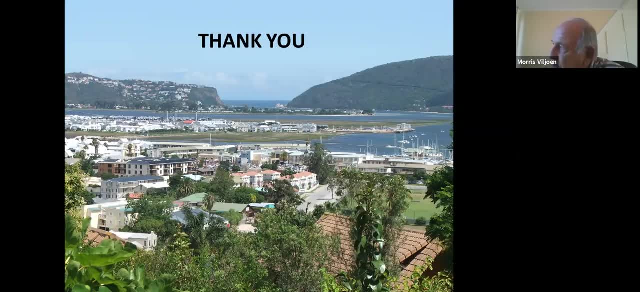 So it's all kind of protected area And but I want to go and speak to the guys at Sandparks here and discuss this whole thing with them And I'm going to take this information and discuss how and work with them and see if they can use it or how they can put it across, because there's a lot of interest in the Sandparks type side of things. 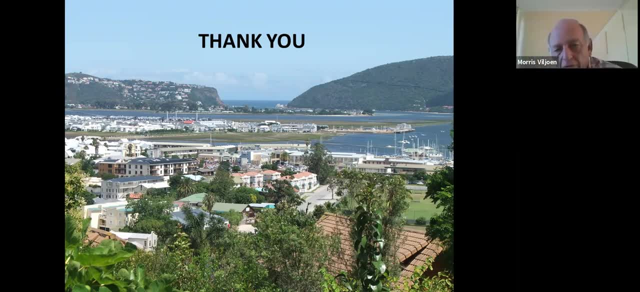 But this could be added to their, to their offering. Yeah, Just a couple more comments from the chat box. Werner says: these are the rocks You're dealing with. there are the equivalent of the Breda's door. Kareem asks Morris. 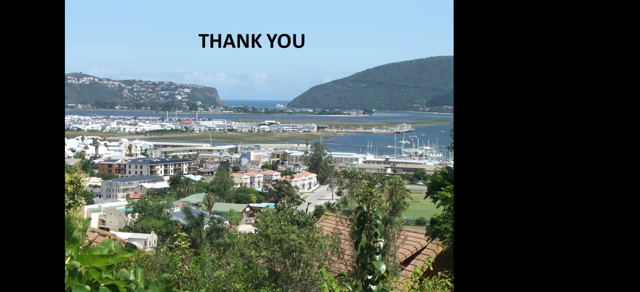 Do you still host day tours to these sites? Yeah, Yeah, Look, I think they possibly are, But I don't know enough about the Breda's door to comment. but I suspect they've got to be. the same processes would have been operating around the whole southern coastline. 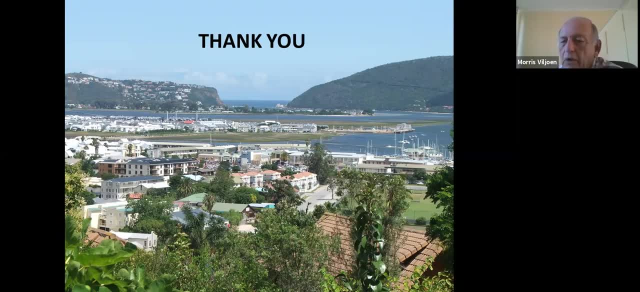 So what I've talked about. I think one could look at the doors and see how you can possibly correlate them, And I think you should be able to, But I don't know enough about Breda's door to comment any more on that. 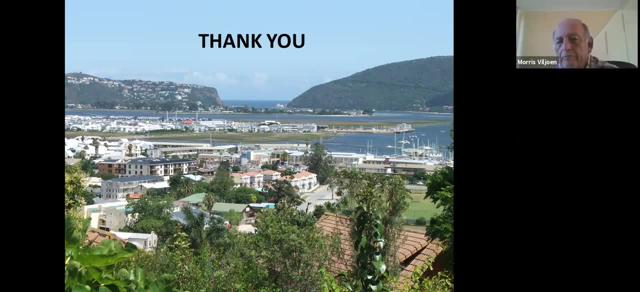 It would be great to have a look at that. And what is the other one about? Do you still run day tours? Yes, Look, I've run tours from both geologists. In fact, one recently was with some high powered geologists. 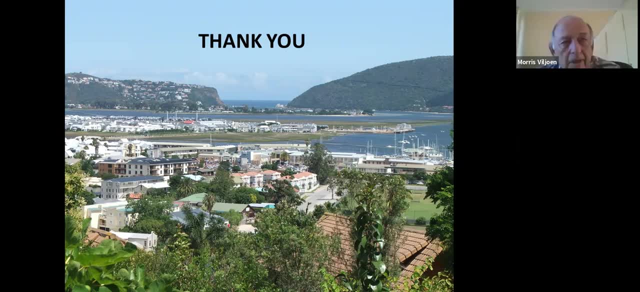 You might know them: Roy Correns, Roger Schoon and Tony Martin from Zimbabwe was here, and a few others. So we had a very good trip down here looking at and discussing all of this stuff, But I've also run several tours with total lay people as well. 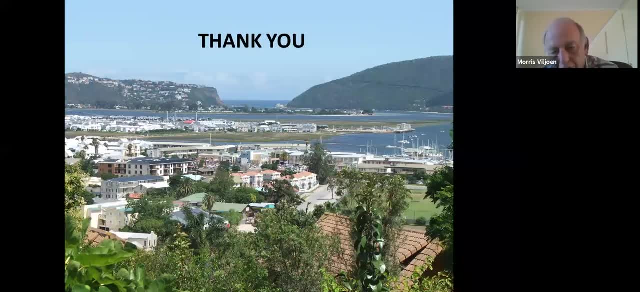 And I'm planning to do a few more of those now that I've got most of this stuff together. What I normally do is I've got a book with A3 color prints of quite a few of these- Well, a lot of the stuff I've shown you. 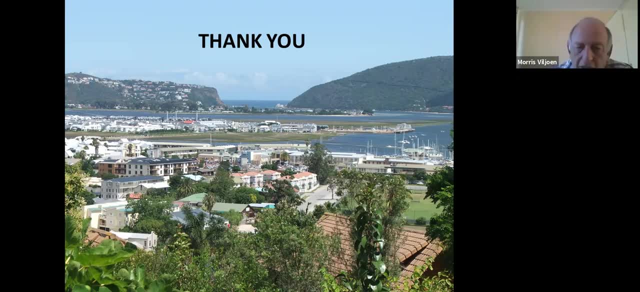 And then color prints of what you see at specific stops, And then I just try and show that and interpret in a very simple way. So that's what I'm. And then also I've got a lady here who's Belinda van Aessen. 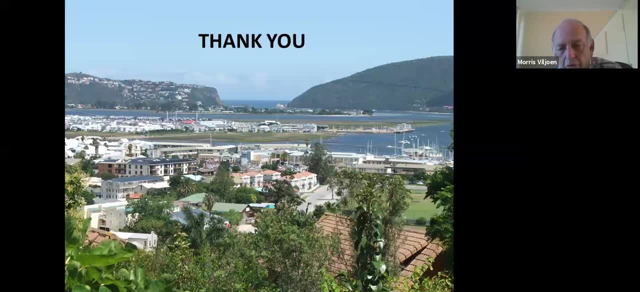 who can do videoing as well. So what I want to do is get a video made of this talk, Get it videoed and have a commentary associated with the video, And also that video can then be used as a virtual tour of this area. 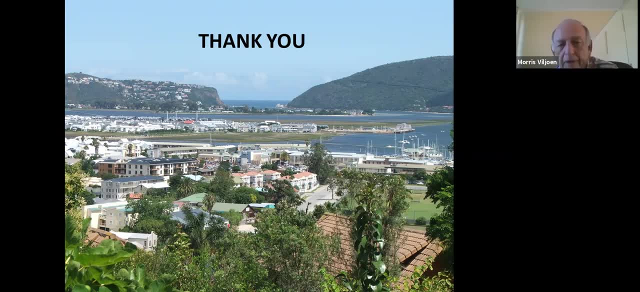 in a video form that people can get hold of. you know, Maurice, you should also find someone with a drone. Some of these features you've looked at, you know, with a slightly higher angle, and a drone will also show up all sorts of things you haven't seen before. 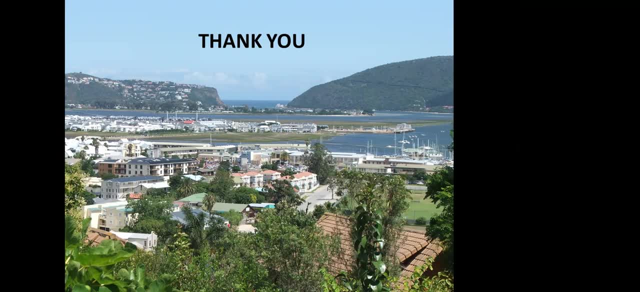 They're amazing, Absolutely right. Yeah, you're absolutely right. And then at some stage we should compare notes- I mean we're doing effectively the same thing with the Overberg group- sort of the long Clarence Drive through Hermanus and the cliff path. 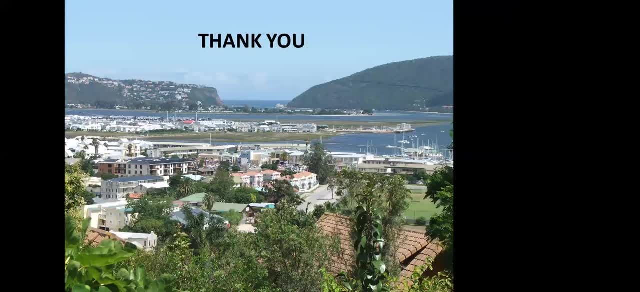 and then round past the Caldas to Gansby And Dave, Dave Morant is quite involved And he's a wonderful resource and just in terms of, you know, dumbing it down, But you know it's surprising, even as geologists. 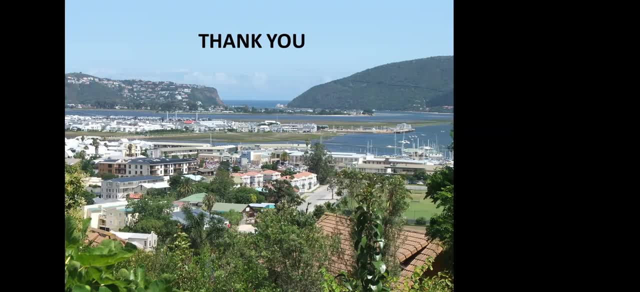 it helps to think simply And suddenly you know we understand things a lot better. Yeah, no, that's right, But I'm glad to hear, And what we'd like to do is any, and we know that there are a lot of people doing their own little thing. 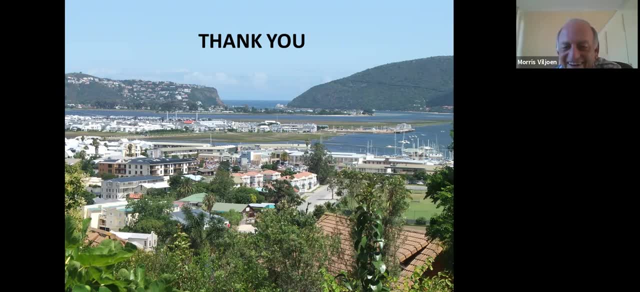 in their own area And guys like Matt Mullins I've heard of just recently and working on the Kuka area or somewhere I think I think it is. And there are many others who have got a passion for certain areas that they know or live in and are doing stuff there. 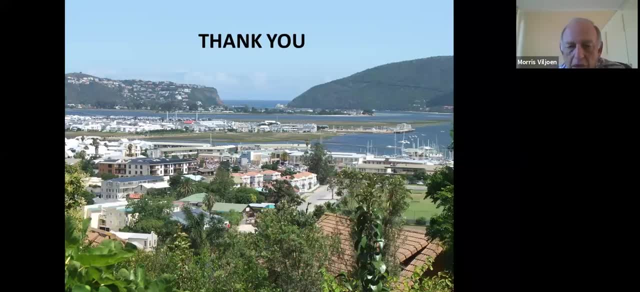 And what we'd like to do- and we're busy with this at the moment- is establishing a platform for promoting geoheritage sites throughout the country, wherever they are, and whoever is doing it, At least make it known so people can you know. 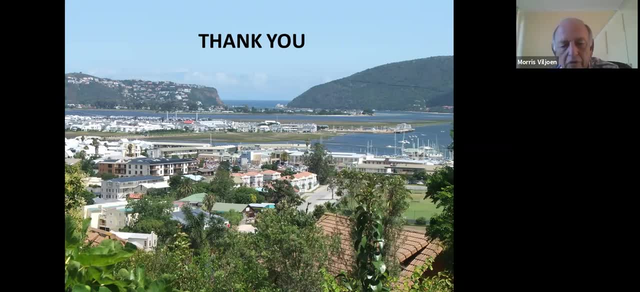 follow up with the people involved and do a tour to those areas And setting up a platform to promote, as I say, all of these activities and initiatives. Yeah, Maurice, I mean again, that's absolutely critical And I've suggested to Craig and the committee that he's got going. 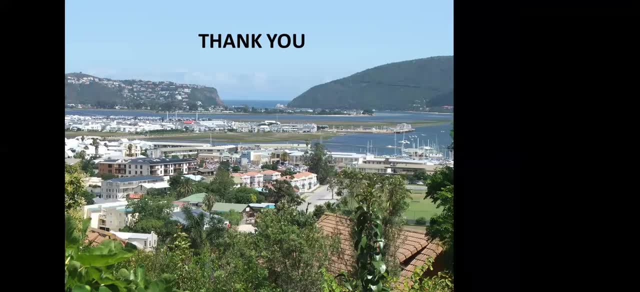 you know we need a register And there's no reason why it couldn't be in the Geo Bulletin, for example, or the website. You know there has to be a register of all this work, which there's a stack of it. 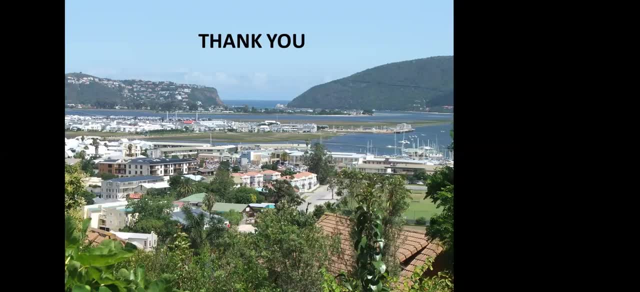 I did send you some of the stuff that's been done on the sort of garden route. I don't know if you had time to look at it. You know, and do yourself a favor, You're not far away. Go and look at the little museum at Prince Albert. 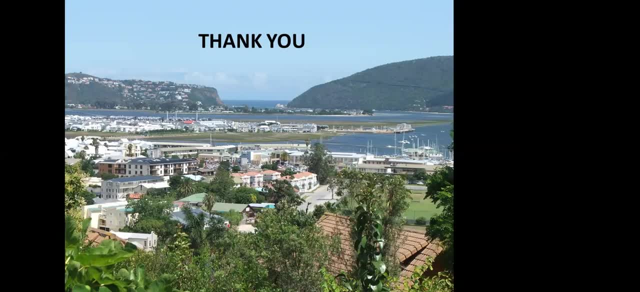 and particularly their rock garden. It's just wonderful And you know rock garden for kids in their stratigraphic column and nice big samples. If they get stolen you can replace them. You can't break it, And then you sort of plant the plant species. 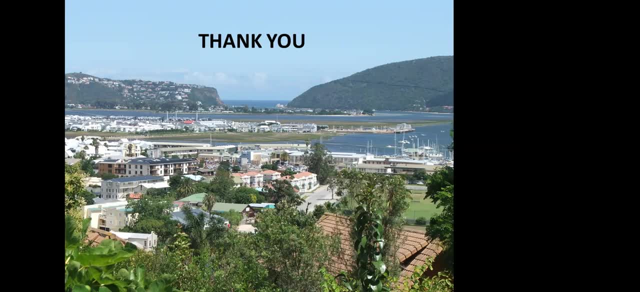 you know, in the gaps between the major geological units The Prince Alfred, Prince Albert Museum is just wonderful. And to add to that, I mean Mike De Witt is doing stuff on Saltpeter Copp and up around Sutherland, So you know. 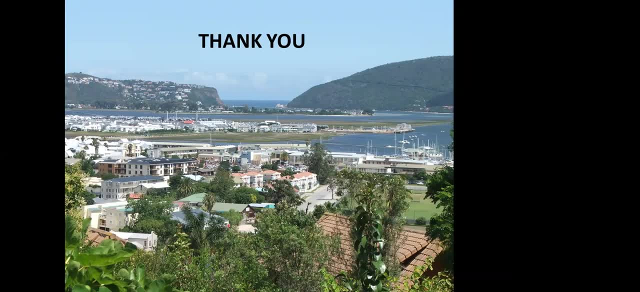 there's an awful lot of work being done, but it needs to be coordinated. And then, Absolutely right, We need a register of all the people doing these kinds of things. So, and then make this available and and and promote their activities and promote. 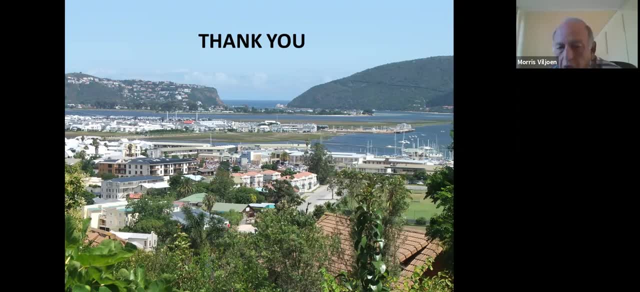 Tours to those areas as well, And, and, either by two operators or even by the, The individual people who might be prepared to do a tour, you know, and in that way popularize science. And, yeah, And, and and geography.